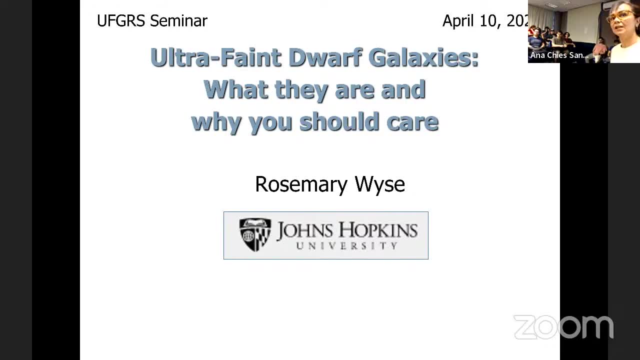 entitled Ultra-faint Dwarf Galaxies What They Are and Why We Should Care. Thank you so much, Rosie. You may start when you're ready. All right, thank you for inviting me to give this seminar. I would, of course, much prefer to be there. 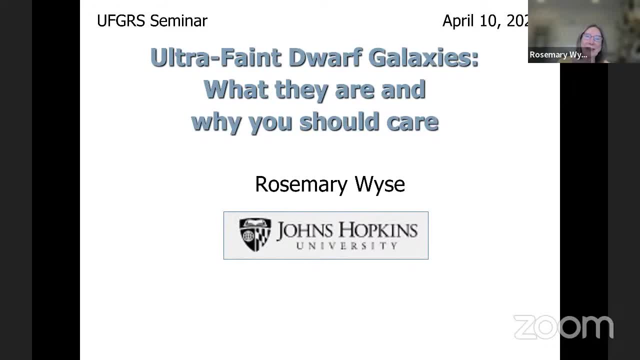 in person and hopefully one day I will manage to spend one of my visits with you in Brazil. So most of my career I have devoted to galaxy formation and evolution across the range of galaxy masses. So I have devoted most of my career to galaxy formation and evolution across the range of galaxy masses. 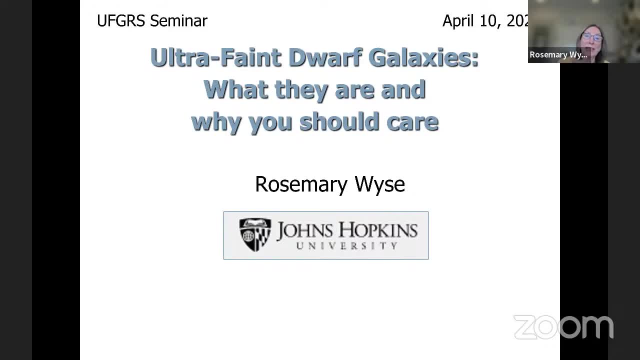 Using both theory and observational techniques, but recently I've become fascinated with the smallest galaxies and I thought I would share with you some of our results, some of the open questions and also what we hope to do with the prime focus spectrograph on Subaru and perhaps 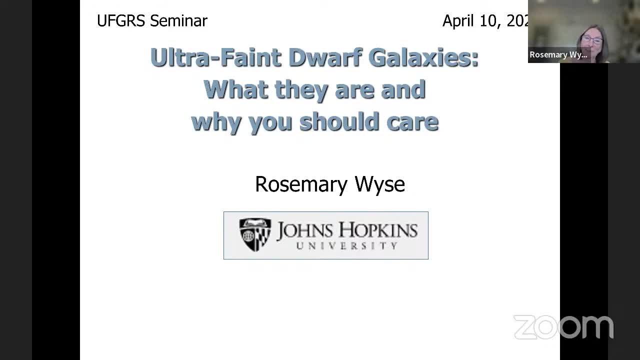 some of you will get more involved with that. So, um, I understand that among you listening we have undergraduates and graduate students, so I will give an overview and I'll be reminding you of results from stellar evolution and other physical processes that are important to how. 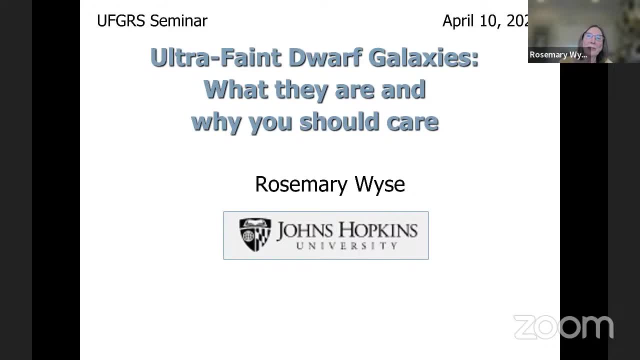 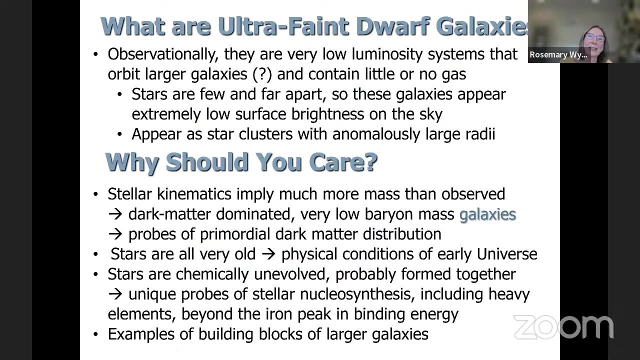 galaxies evolve, So I hope that those are helpful for you. Thank you so much to all of you who have you, who are experts in the field, will be patient with me at that point. So, just to get us going, I'll tell you what I'm going to tell you and then I'll tell you it. So the first important question. 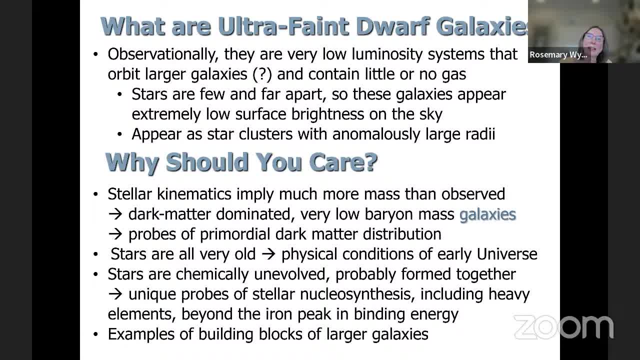 the part of my title. what are ultra faint dwarf galaxies? Well, observationally they're extremely low luminosity systems. They tend to be satellite galaxies of larger galaxies. I've put a question mark there because just recently there have been two new discoveries of extremely low luminosity. 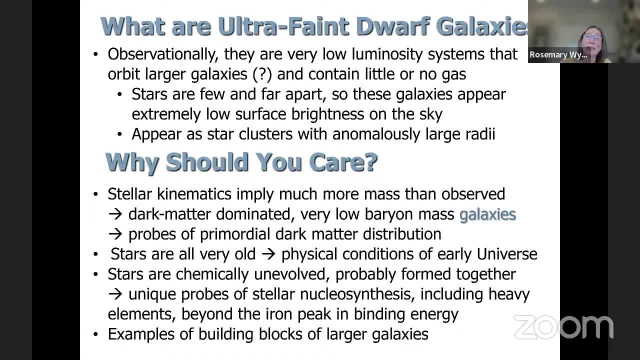 systems that we think are galaxies that are actually between the Milky Way and M31. And it's not clear that they're in orbit about either large galaxy. But the vast majority of ultra faint dwarf galaxies are satellites of other larger systems. They seem to contain just stars, at least. 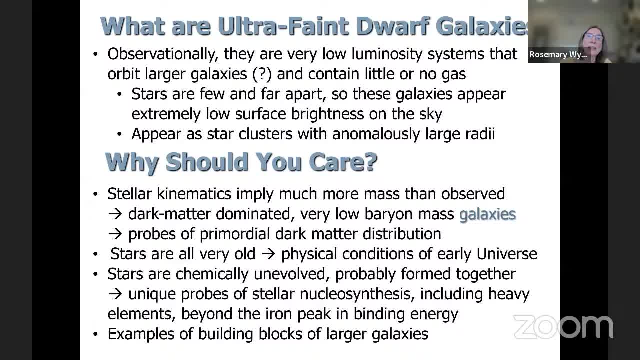 observationally, There's little, No gas. The stars that they do contain there's very few and they're quite far apart, So they're extremely low surface brightness on the sky. They've been detected so far by a slight over density in star counts basically, So they appear like star clusters, but with much larger radii. 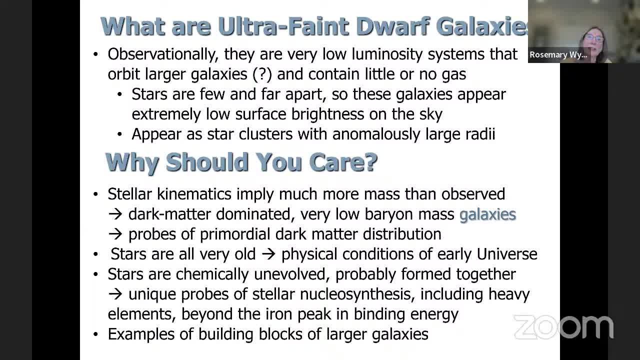 than would be typical for a star cluster. So what's the importance of these very small systems? Well, the first aspect of them that, I think, sets them apart is that, even though they have very low luminosity, they contain much more mass than is observed in the stars, And indeed, 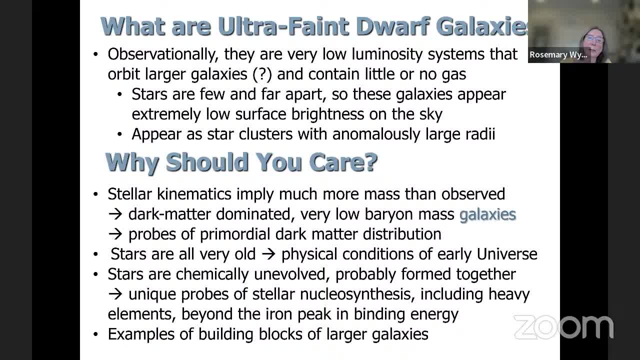 they're among the most apparently dark stars. They have a very low luminosity and so they're among the most apparently dark matter dominated systems in the universe. They're very dark matter dominated. They have a very low baryon content, just a few stars. 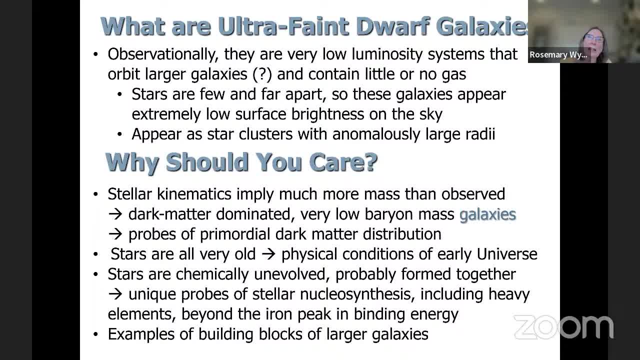 So that means that they have a low enough baryon content that it basically hasn't disturbed the distribution of dark matter. And we'll see later that in more luminous galaxies the baryons can actually change the distribution of dark matter. So that means with these ultra faint, dwarf galaxies, 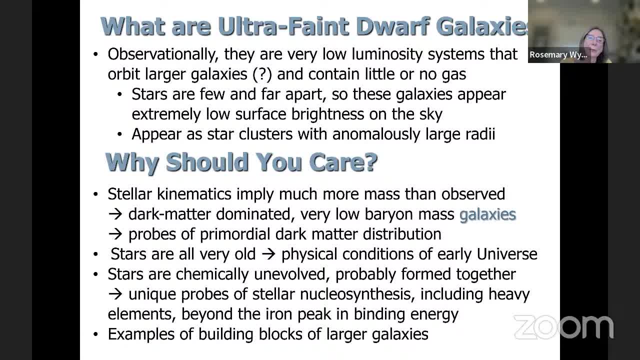 if we can determine the distribution with radius of the dark matter. that's telling us what the dark matter itself wants to form as the density distribution. That's what I've referred to as the primordial dark matter distribution, And that depends on what the dark matter is. 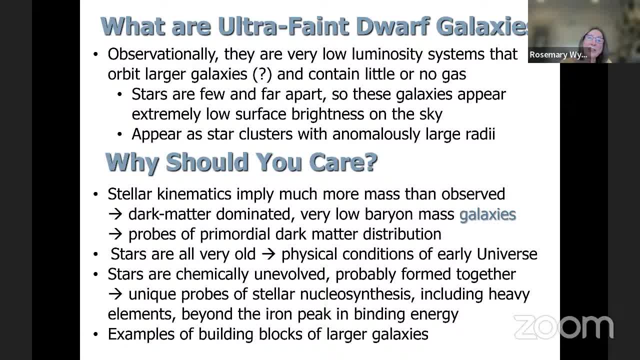 So that's very important. The stars that are in the ultra faint dwarf galaxies all seem to be extremely old. That means they formed at very large look back times. So when they formed it was very, very early on in the evolution of the universe. 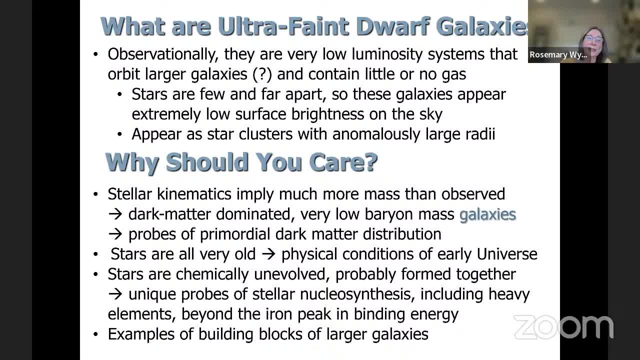 So they're probes of the physical conditions at high redshift. They're very chemically unevolved and they probably all formed together in the dwarf galaxy And they're unique probes of stellar nucleosynthesis at high redshift, And that includes the origins of very heavy elements. 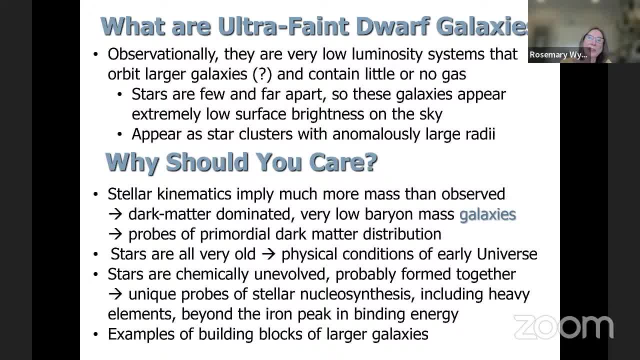 those beyond the iron peak in the curve of binding energy per unit nucleon. We live in a large galaxy. in our current paradigm of cluster of galaxy formation, predicated on the dark matter being cold dark matter, We start with small systems which merge to form large systems. 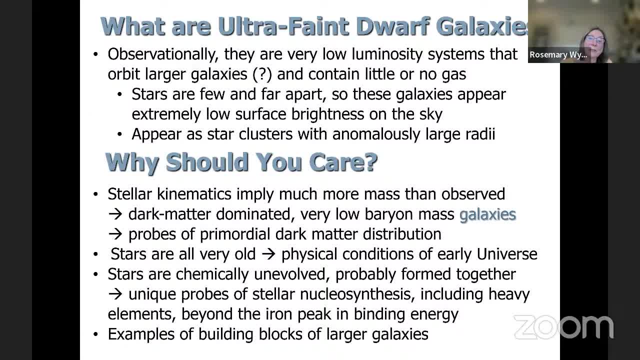 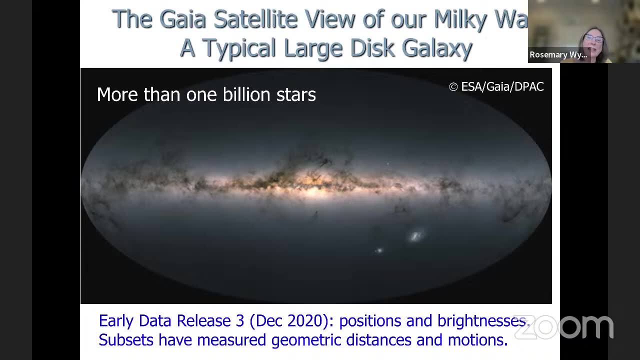 larger systems And these ultra faint dwarf galaxies are plausibly examples of building blocks of larger galaxies. So for all these reasons, you should care. So now let's explore in more detail some of these aspects of dwarf galaxies. But first for context. 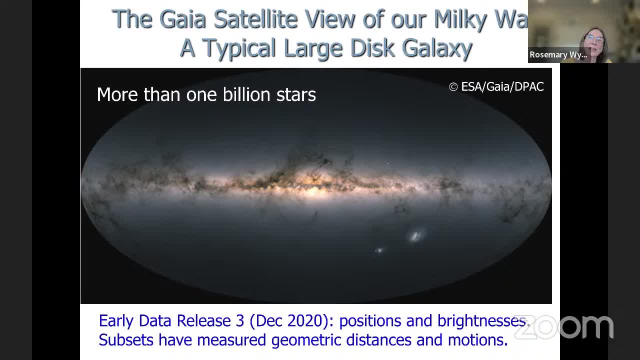 let's consider our galaxy, which is a typical large disc galaxy and the field of study of our Milky Way, commonly referred to as galactic archaeology, Also near field cosmology, to reflect this idea that by looking locally at old stars we can constrain star formation at high redshift. 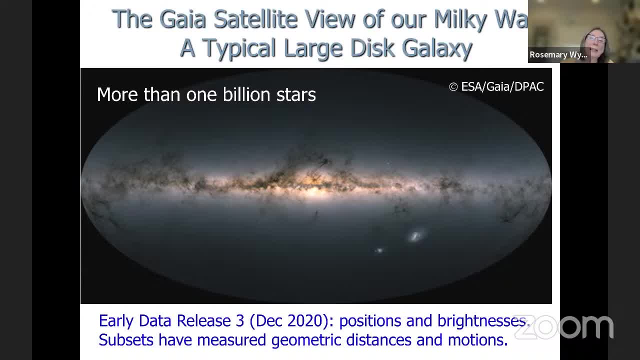 The cosmological look, the size of the stars. that field has really been transformed by the ESA satellite, astrometric satellite Gaia, and here's just a view of more than 1 billion stars in our galaxy And you can see. most of them are in the disk. 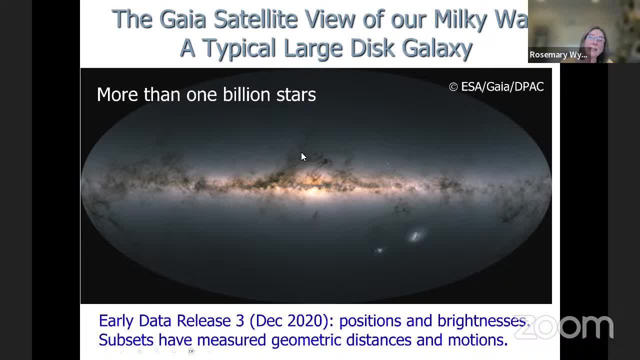 we have the bulge in the center of the image. here In the center of the image, the bulge is the center of the image of the galaxy, center of the galaxy. This galaxy, the stars and dust are concentrated to the disk. 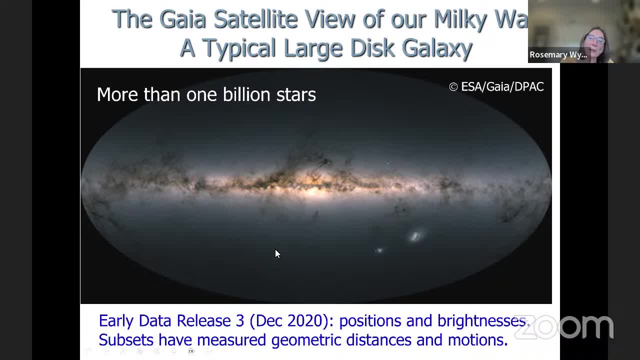 And let me just point out to you here there is a tiny globular star cluster. So there are stars very far from the disk. We have a globular cluster here, just stars. We also have two satellite galaxies, the Large and Small Magellanic Clouds. So galaxies have star clusters far from the center. 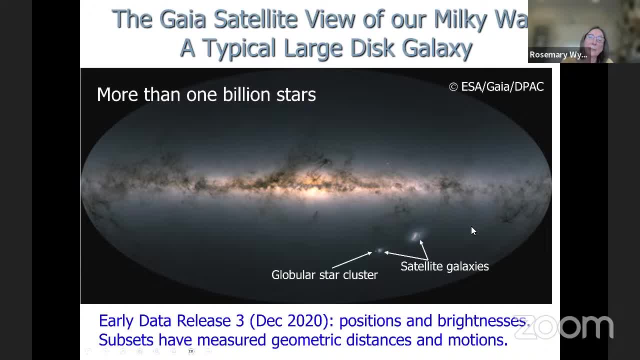 and they have satellite galaxies far from the center. Of course, although this globular star cluster and the galaxy are very close to each other, they are not very close to each other. So galaxies are together on the sky, they're at different distances, And one of the important 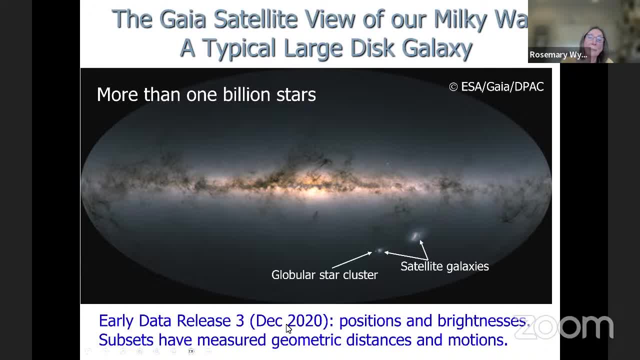 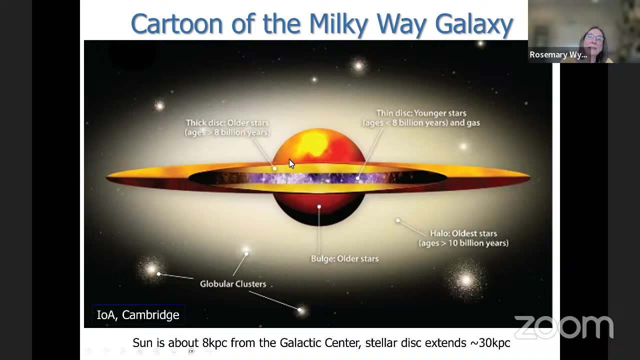 aspects of Gaia satellite was that it measured geometric distances for millions of stars in our galaxy and beyond. So we have a cartoon of the Milky Way galaxy. We have the bulge, older stars, the stars. We have the thick disk which I worked on a lot in the 80s and 90s, establishing those stars were old. 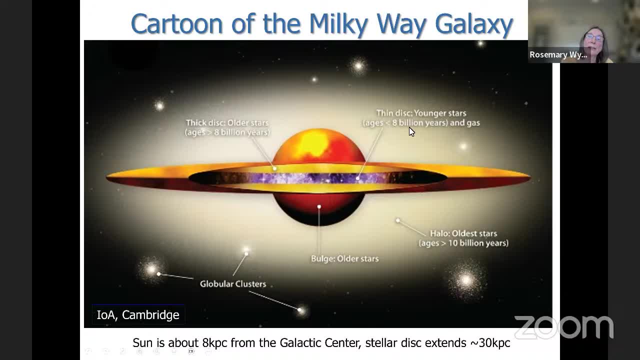 The thin disk where stars are forming, younger stars, including up to zeros, since stars are forming there now And we have this halo, the oldest stars, where we find these globular star clusters. So to set some sort of a map of the galaxy. we have these globular star clusters, So to set some 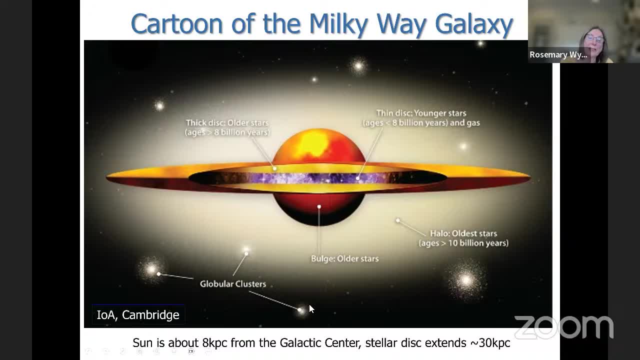 scale here. the sun is about eight kiloparsecs from the galactic center. The stellar disk extends about 30 kiloparsecs from the galactic center. Thin disk stars are on close to circular orbits about the center, high angular momentum, Halo stars, including the globular clusters. 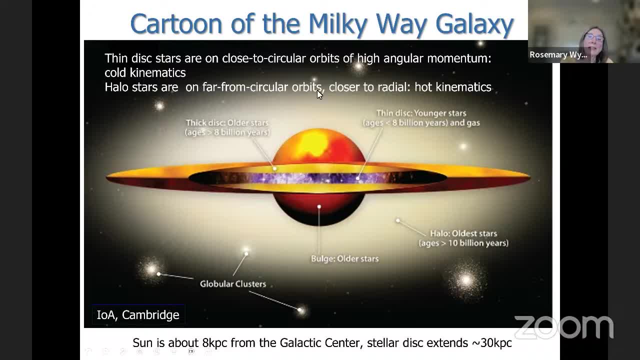 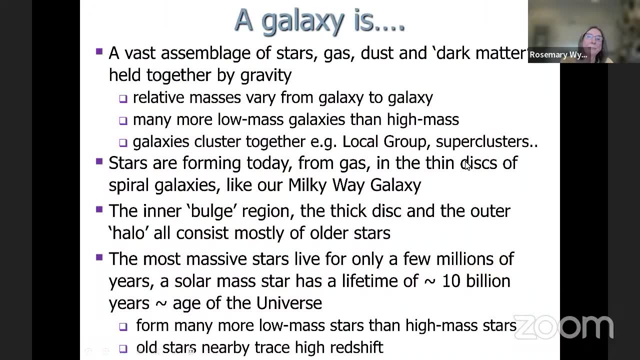 and in general, including satellite galaxies are on far from circular orbits, which we refer to as hot kinematics. So I'm going to go through why we think ultra faint systems could be galaxies. So let's just think about what is the definition of a galaxy. It's a vast assembly. We have stars and we have 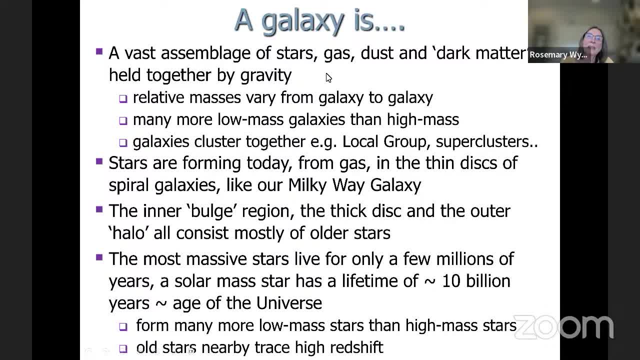 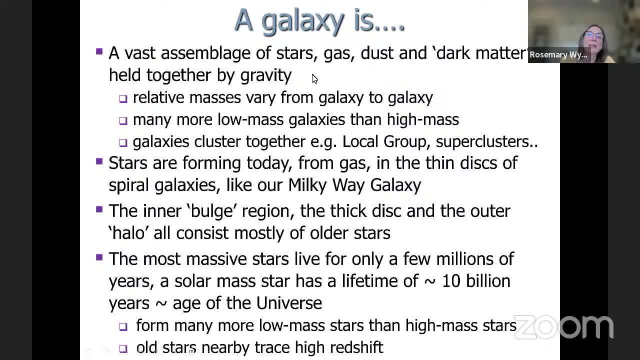 gravitational field is dominated by the dark matter. The relative fractions of stars and dark matter- stars to dust, etc. varies from galaxy to galaxy, And nowadays there are many more low-mass galaxies than high-mass galaxies, And galaxies cluster together. We have the Milky Way and its 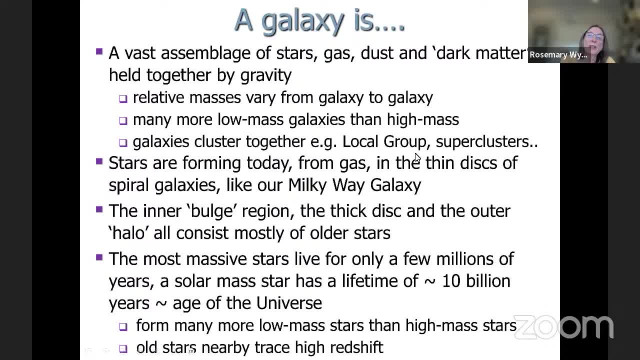 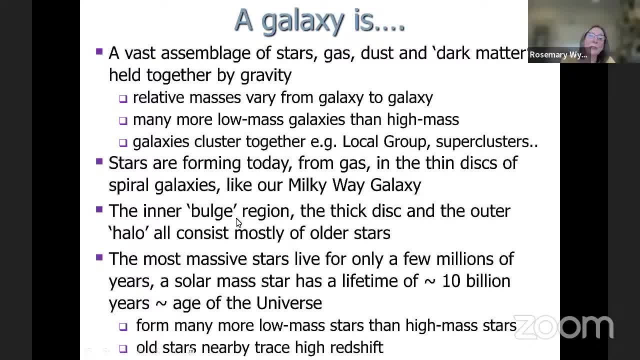 have stars, gas, dust and dark matter, And we have galaxies And we'd like to know what makes stars form, where they formed. What are the properties of stars? How did star formation differ if it did at early times than it does now? To probe early times, we take advantage of the 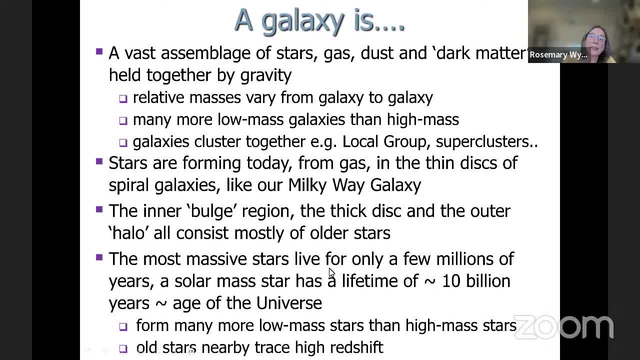 fact that, even though the most massive stars live for only a few millions of years, A star of order- the mass of the sun- has a lifetime that's much longer, of order 10 billion years, which is, of order, the age of the universe. 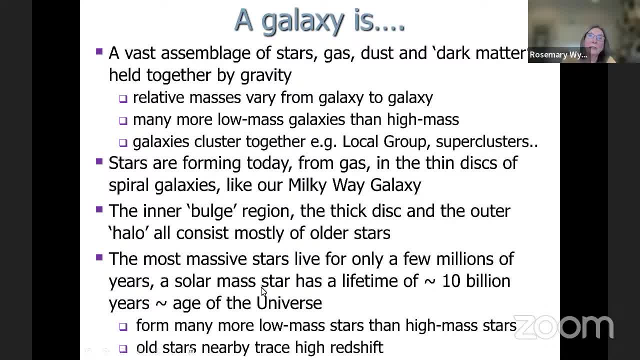 So if a star of the same mass of the sun or below formed 10 billion years ago, it's still around now. So all the stars nearby trace conditions of high redshift. redshift, sorry. 10 billion years is about 10 billion years ago is about redshift of two. 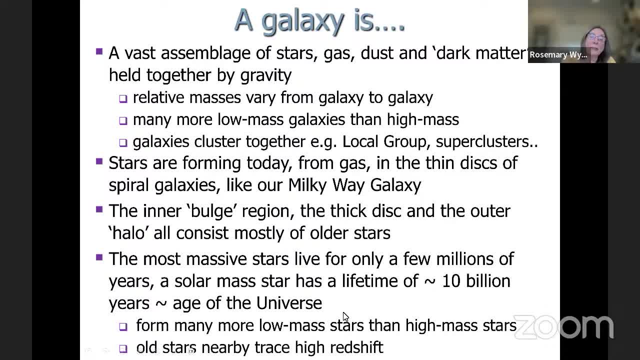 And the way star formation, I would say, operates, or the way stars form. there are many more low mass stars in a bird's eye view. So we have many ancient low mass stars nearby that we can study. So I mentioned satellite galaxies of the Milky Way. 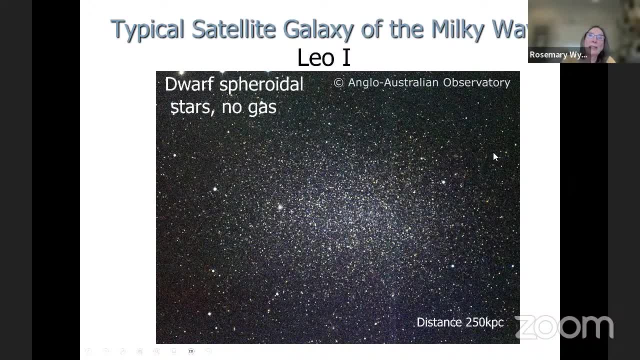 I pointed out, to the large and small Magellanic clouds. Those are quite massive for satellites and have a lot of gas and ongoing star formation. They're actually not typical Satellites are. more typical Satellite is like this one here called Leo one, the first satellite found in the line of sight where the Leo constellation. 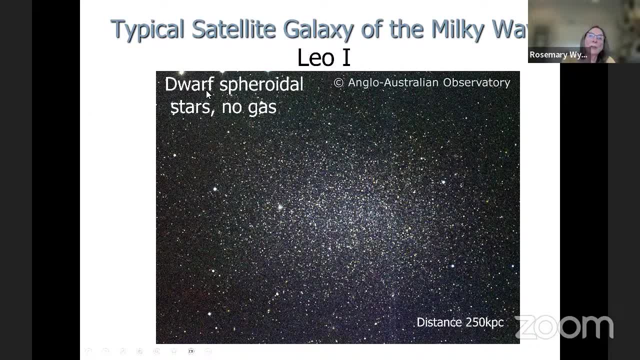 This is we refer to as a dwarf- spheroidal. dwarf meaning low luminosity. spheroidal meaning it looks sort of spherical on the sky. It consists, observationally, of stars And no gas. This one is at a distance from the center of the galaxy of about 250 kiloparsecs. 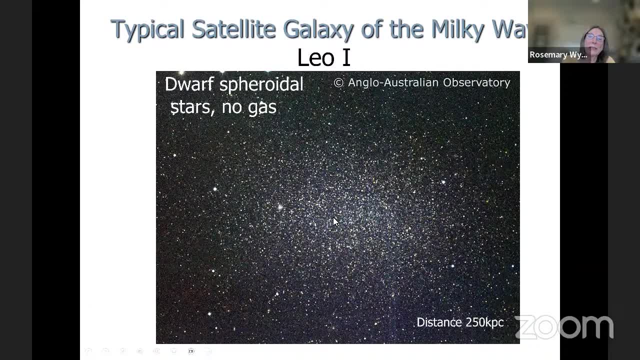 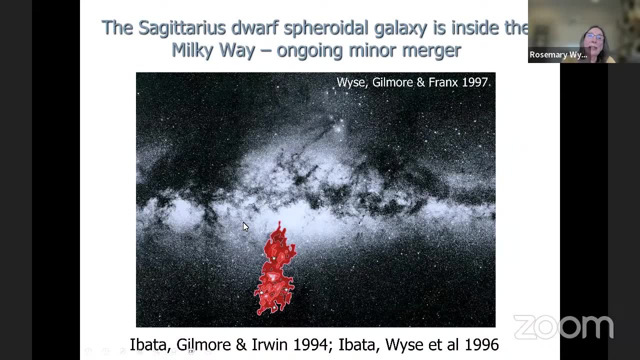 So almost 10 times the extent of the disk of the galaxy. We do see dwarf galaxies more nearby. In fact we see one inside the Milky Way. There's Sagittarius dwarf spheroid. Sagittarius dwarf spheroid. 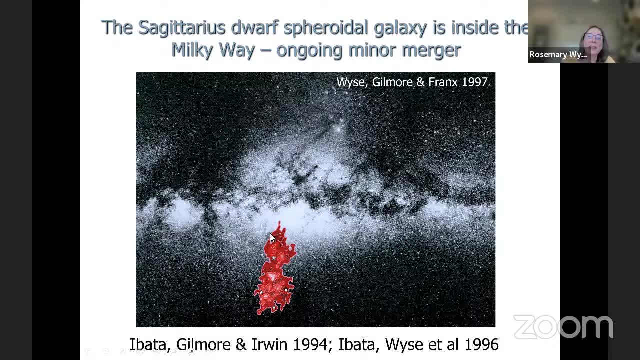 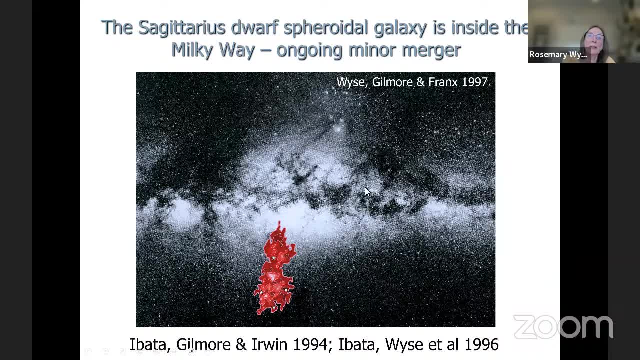 It's shown here projected against the bulge of the galaxy, but it's actually on the other side and it's on an orbit coming up. It's shown here projected against the bulge of the galaxy, but it's actually on the other side and it's on an orbit coming up. 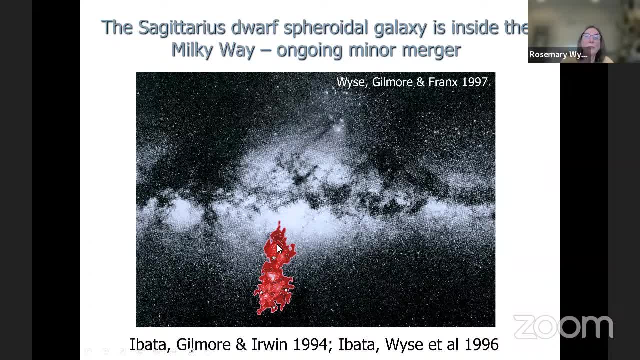 From having done a circuit around the center of the galaxy, it's coming up, It's being stretched out due to tides, the gradients of the gravitational field of our galaxy, And this is an ongoing merger of a satellite galaxy, one of the building blocks of bigger galaxies, into our galaxy. 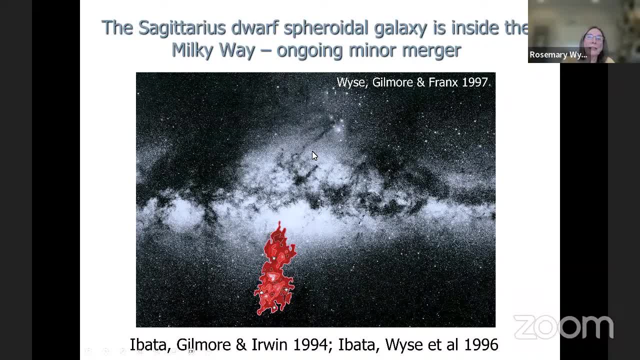 And this is an ongoing merger of a satellite galaxy- one of the building blocks of bigger galaxies- into our galaxy. Stars will be lost from it and it will be assimilated into our galaxy. This dwarf galaxy was discovered by Roddy Ibata and Jerry Gilmore during their survey of the central bulge of our galaxy. 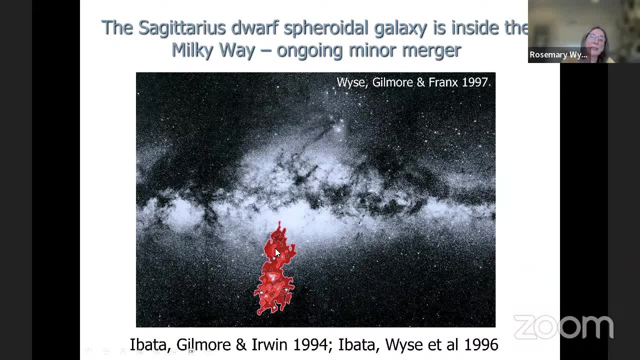 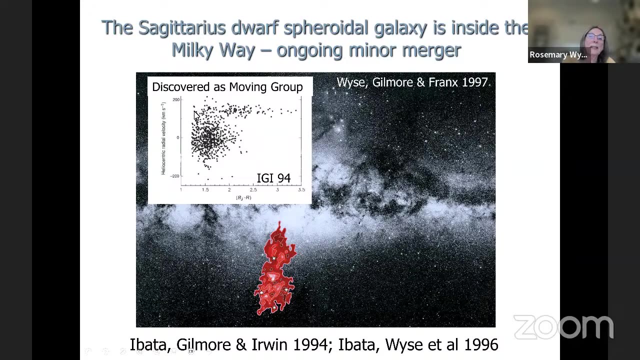 They had spectroscopic fields around here, some crossing this area of sky. Mike Irwin then mapped out the extent of a system that matched the properties of the moving group that they found as part of their spectroscopic survey of the bulge. They found stars that all seemed to be moving together but were not moving. 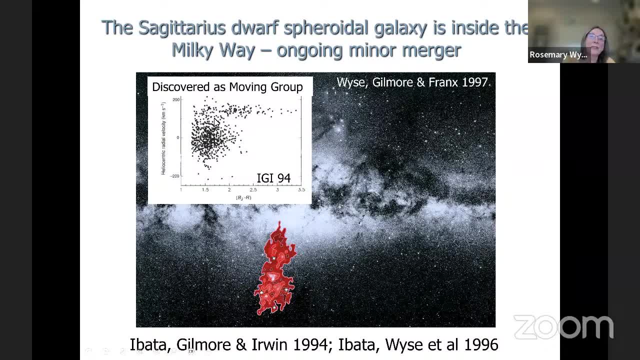 Similarly to most of the other stars at the center And they then found. also the colors of the stars were different from the bulk of the stars in the center. So satellite dwarf galaxies can be found from their distinct color magnitude diagram and then confirmed as galaxies by getting kinematics. 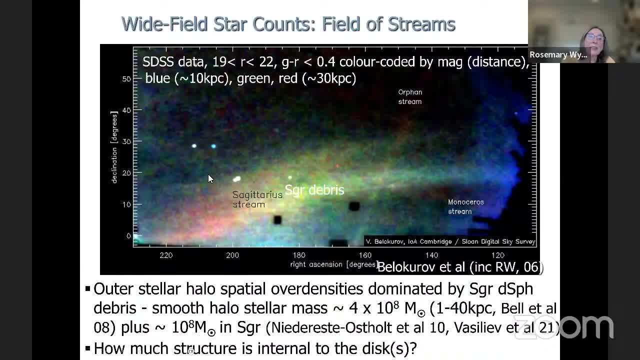 We now have much better wide field imaging surveys and we can see that the Sagittarius dwarf is being tidally disrupted by the Milky Way and debris from it are seen across the sky. This is a figure taken from Belukarov et al of star counts in the slow motion. 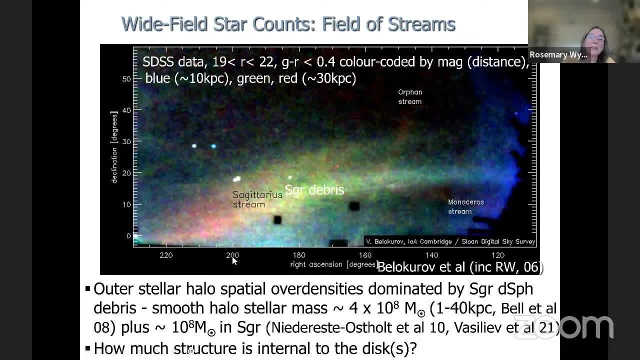 This is a figure taken from Belukarov et al of star counts in the slow motion. We have a full-angle drone Digital Sky survey. this is a wide area across the sky. Well, starting at the Equator, we see 60 degrees of declination from zero up. 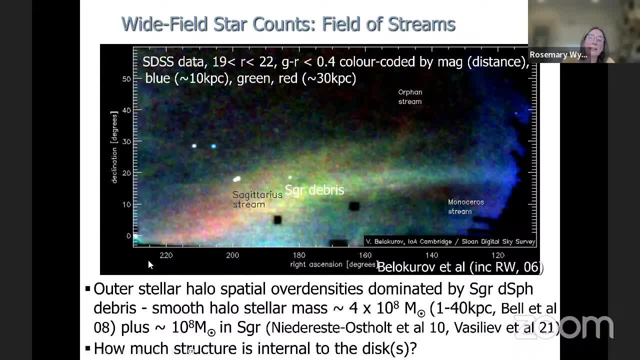 And we have 60 degrees of declination and angle on the sky. Again, We have about 100 degrees here. What I hope you can see, The stars here are faint stars. this is the apparent magnitude and the R band and they're. 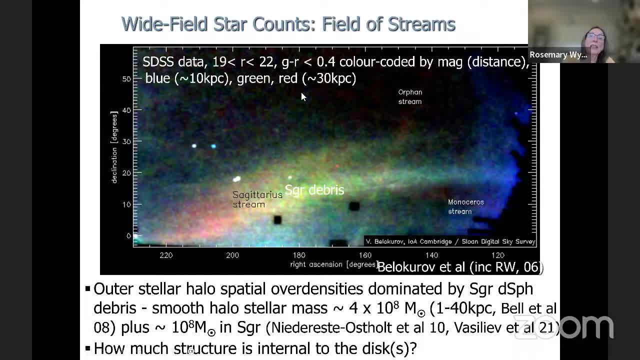 colored. they're bluish stars and they're color coded in this plot by their apparent distance. they're color coded by their apparent magnitude. the stars are all similar: main sequence stars, dwarf stars. so color coding by apparent magnitudes, color coding by distance, what you can see. 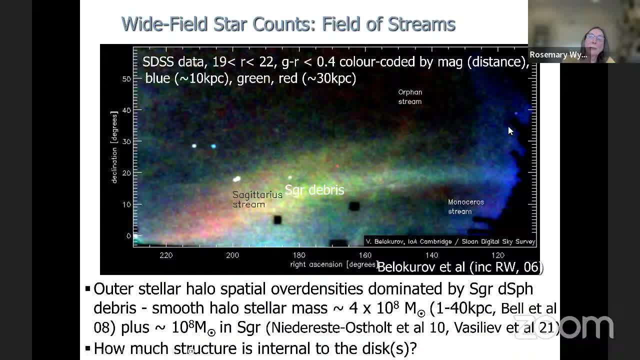 is blue is nearby. there's a blue swath here, green intermediate distance, about 20 kiloparsecs away, again a swath, all at the same distance, and then red being more distant again. so it's far from uniform on the sky showing us debris from satellite. 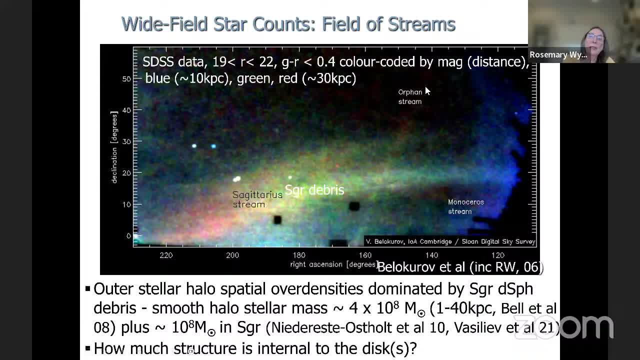 systems that are being tidally disrupted. we have the orphan stream streams from the Sagittarius Dwarf and what was referred to as the Monoceros stream, so this image was referred to as the field of streams. the Monoceros stream was thought to be. 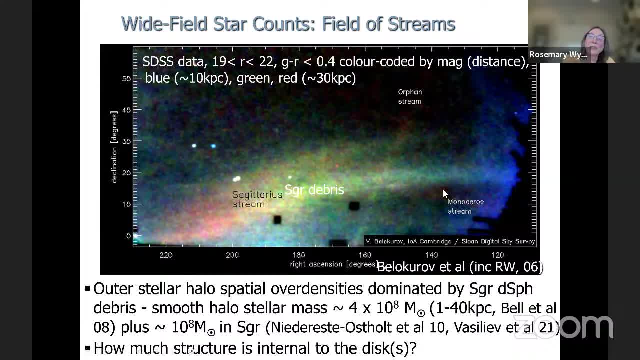 it's in the anti-center direction. this is towards the outer disk of our galaxy, and it was thought to be a disrupted satellite. The question was: is it a satellite or is this structure in the disk? And we now have got better data- spectroscopic data. 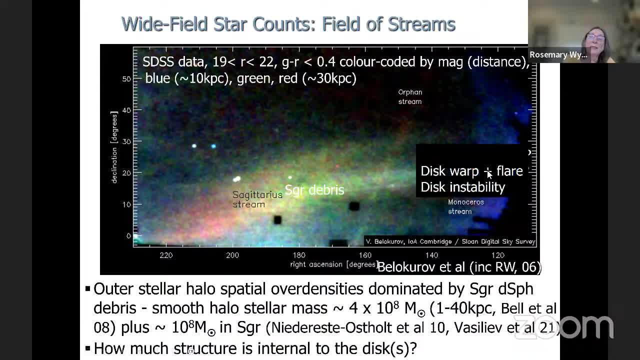 and this is structure in the outer disk. What you can see is written here. the outer halo is dominated by spatial overdensities that are dominated by the Sagittarius dwarf. It's about equal mass in stars from the Sagittarius as there is in the smooth halo and a 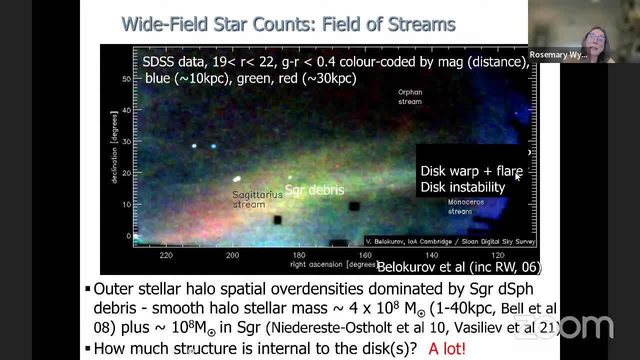 lot of structure towards the outer part of the disk is actually internal. A lot of work from Gaia. But let me turn to the main topic of my talk. This is not just the field of streams, it's the field of streams and dots. There is a little red dot here. 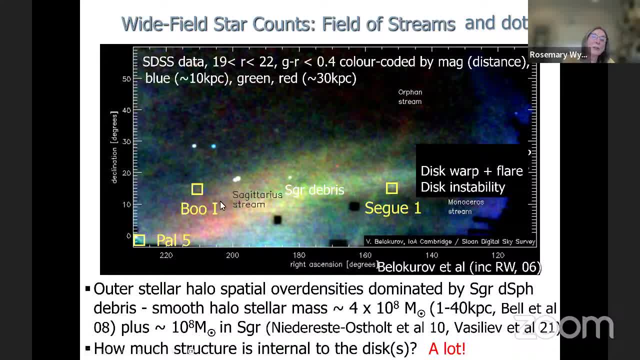 that's stars from the Boötes dwarf, spheroidal, ultra faint dwarf we now know is another little dot here. These are stars, spatially coincidental stars. These are stars spatially coincidental stars. These are stars spatially coincidental stars. 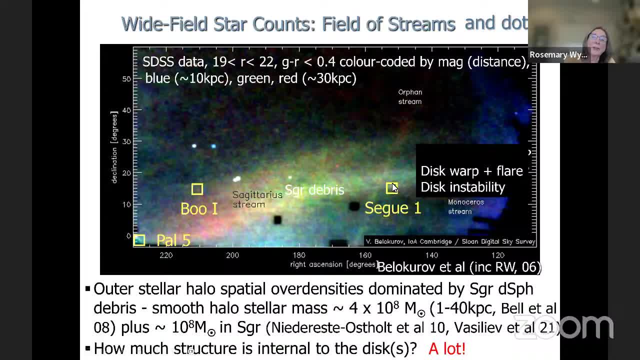 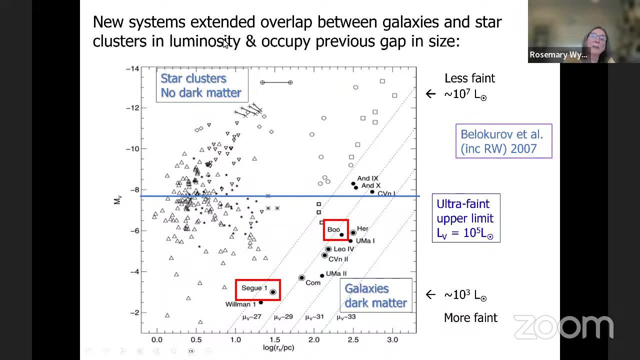 And in distance, and also on the sky. these are clusters of stars. Down here there's also a dot with a stream. This is Palomar five, a globular cluster in our galaxy. So these new systems, these ultra faint dwarfs, 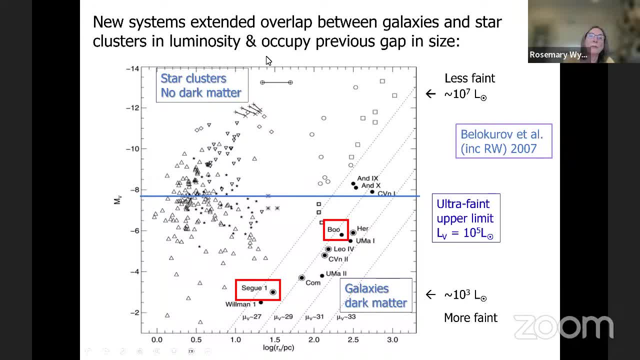 that were first discovered due to the uniform photometry that Vassily Belukharov created for the Sloan Digital Sky Survey. they overlap in luminosity between galaxies and star clusters. This is a plot of absolute brightness of a system versus the half light radius. 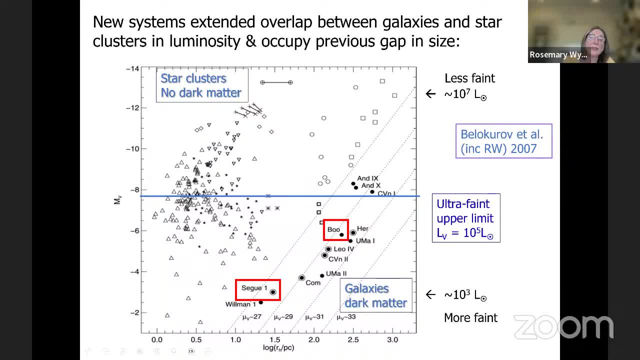 a measure of the concentration, the size of the object. The left hand side is the star cluster, The right hand side are star clusters. I mentioned a galaxy has dark matter. star clusters, as far as we know, have no dark matter. 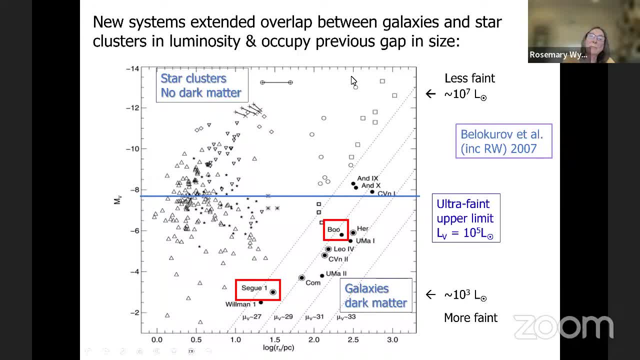 They're held together by just the gravity of the stars. The right hand side we have dwarf galaxies. The brighter systems were known to have dark matter Before the discovery of so. most star clusters are fainter than about 10 to the five times. 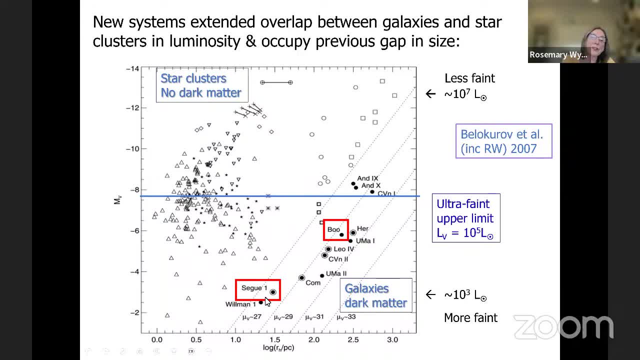 the luminosity of the sun And before the discovery of these very faint systems, there was a gap in radius between star clusters with no dark matter and dwarf galaxies And the dwarf, the star clusters. they're not very faint, They're not very faint. 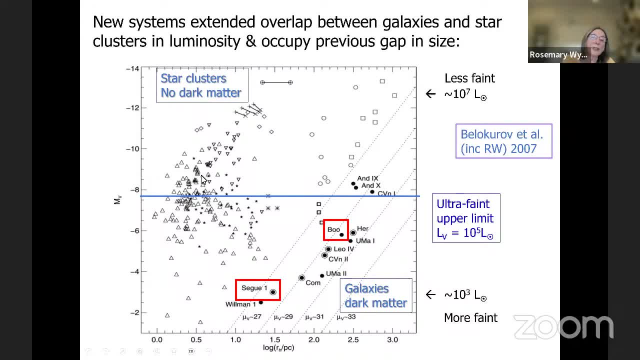 They're not very faint, they're not very dark, But they do have a more interesting range of luminosity than a star. here The star clusters- And the star isn't there. The star cluster range of luminosity is extended, much fainter than the dwarf galaxies. 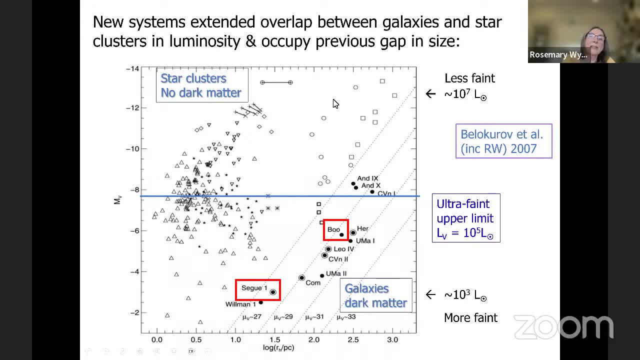 But these new systems extended the overlap between star and star clusters and dwarf galaxies and luminos. Today there's no longer a distinction, And there's also no longer a distinction in sight. I've been thinking about this, So they're very strange. 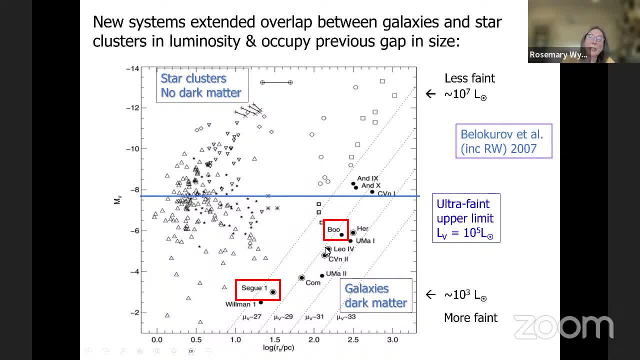 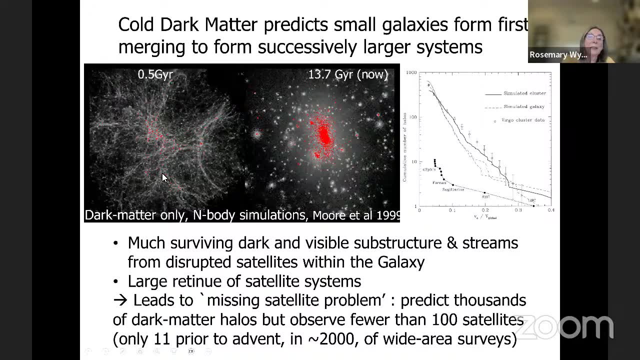 How do we know that these systems are galaxies? Well, we expect to have lots of very faint galaxies. If we have a system where dark matter that controls the gravitational field is cold, then I have very small systems forming first and they merge to form large systems. 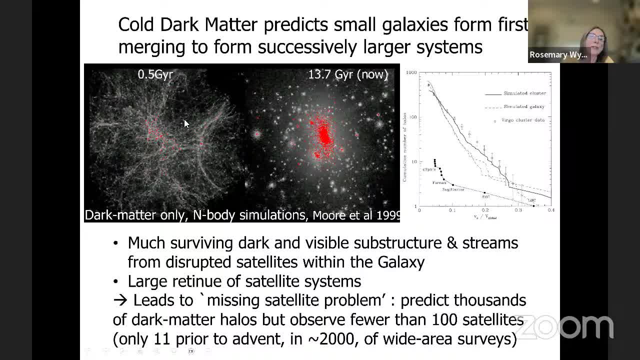 just shown here in two snapshots, very early times over dense regions. self-gravitating regions of dark matter are labeled by red here the most dense systems at early times likely to form stars clusters together to now, And you can see lots of the gray, is dark matter only. 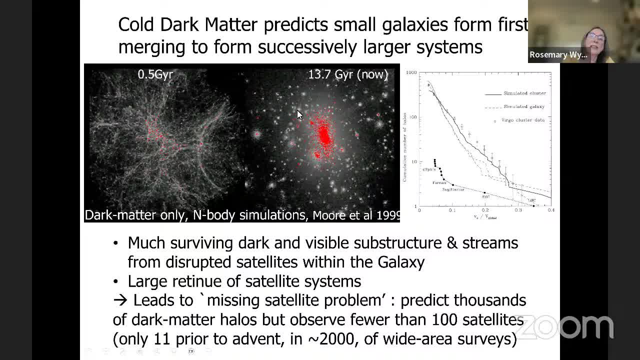 Again, the red is where we think stars likely formed. We have luminous dwarf galaxies, many of them predicted, and also many dark systems, And this led to what was referred to as the missing satellite problem. There are many more predicted, even luminous, small dark matter halos than observed satellites. 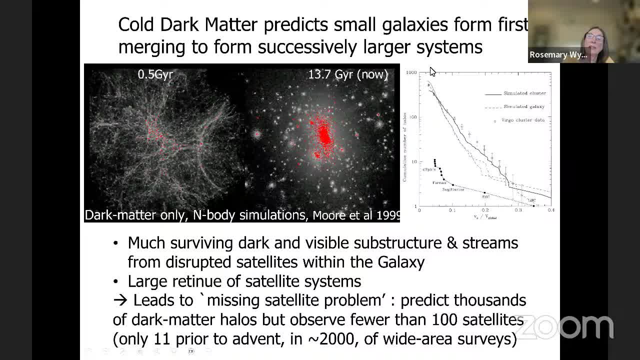 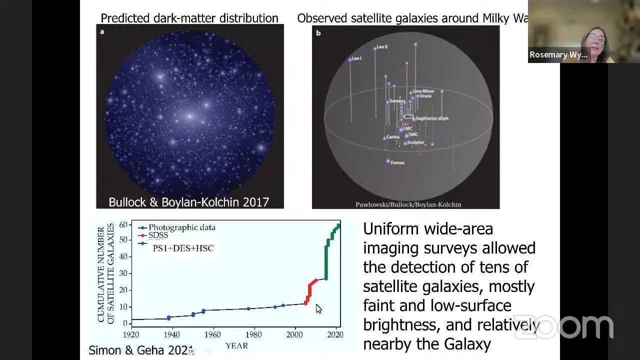 And this is just an example here of predicted This is dark halos, but many of these should have stars and the dwarf spheroidals. Of course. as we have better and better surveys, better techniques to find satellite systems, we're finding more of them. 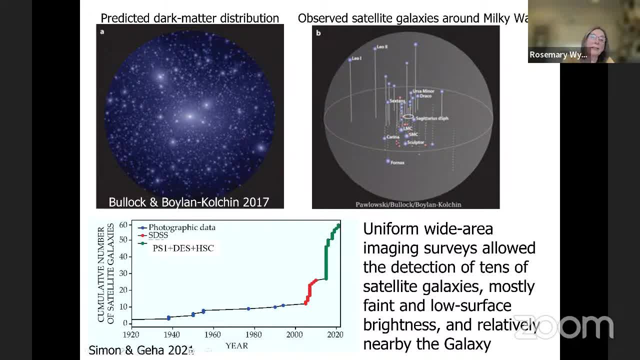 Here's just a figure from Simon and Geha in 21.. This back here was 99, to show you the progress that we've made since Sloan. and then Pan-STARRS, Dark energy survey and hyper supreme cam were finding more and more dwarf satellites. 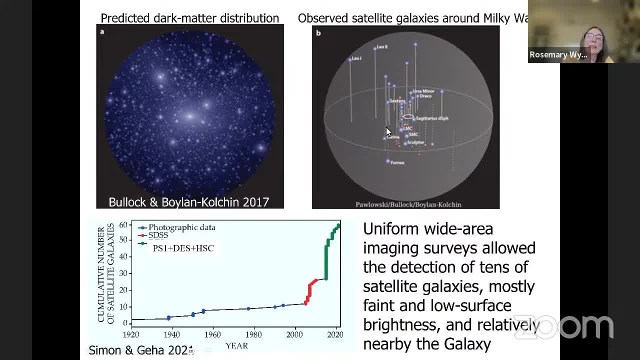 But we're still not at the predicted distribution and luminosity function predicted by cold, dark matter. But of course we're all looking forward to the Rubin satellite, The Roman satellite and the Rubin satellite LSST survey, expected to find many more dwarfs. 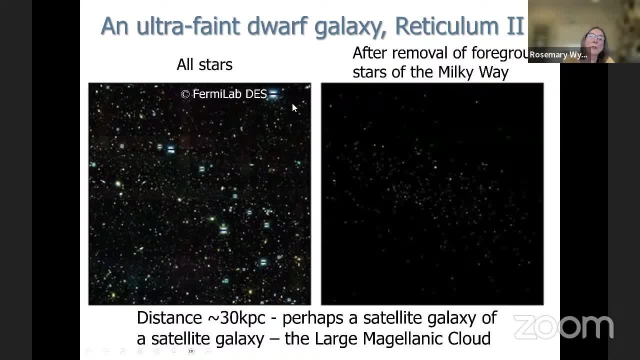 One of the new dwarfs that was discovered by the dark energy survey just shown here. This is a snapshot taken from the dark energy survey page. This is an area of sky, quite a few stars here, But if you remove the foreground stars of the Milky Way. 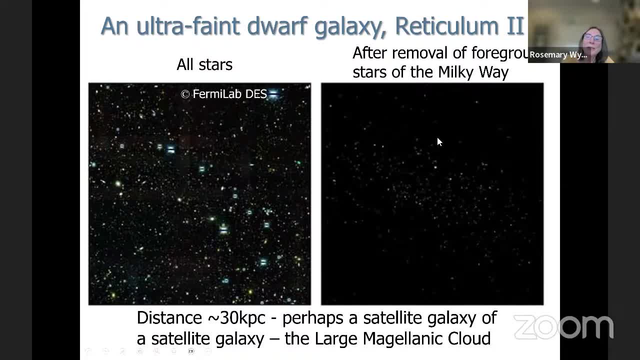 there's a few stars visible here, And that's the galaxy called Reticulum 2 that I'll be returning to later. It's particularly interesting because this could be a satellite that's going to be in the Milky Way. This could be a satellite galaxy of the Magellanic Clouds. 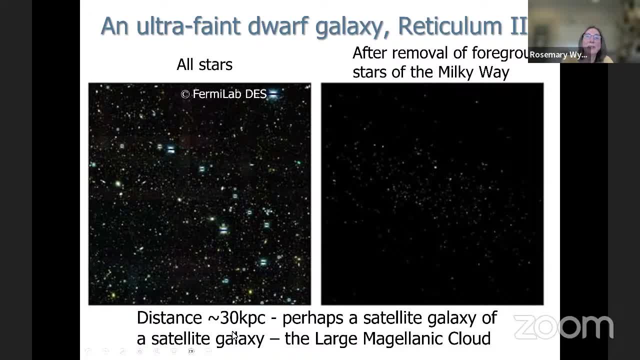 the Large Magellanic Cloud, which itself is a satellite galaxy of the Milky Way. So again we have hierarchical clustering satellites of satellites And of course we'd like to, before we leave, we'd like to know was star formation, chemical evolution, et cetera. 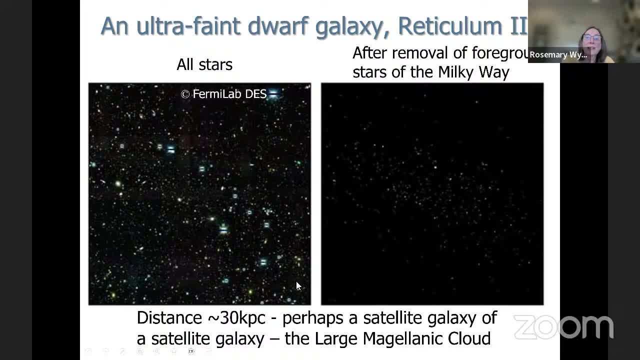 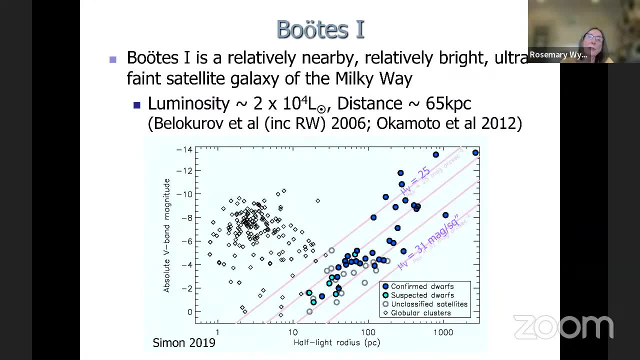 any different If you're a satellite of a small galaxy or a satellite of a large galaxy. I'm going to focus most on Boötes 1 for two reasons: It's relatively nearby and it's relatively bright as far as ultra-faint satellite galaxies go. 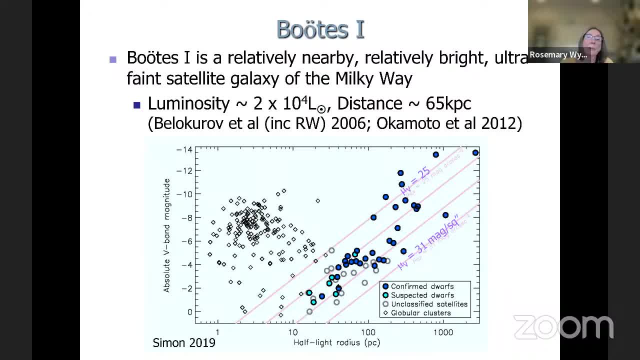 Its luminosity is close to the kind of working definition of ultra-faint, which is less faint than 10 to the 5 solar luminosities. Its distance is actually about 60 kiloparsecs. Here's an update of that plot I showed of absolute magnitude or luminosity. 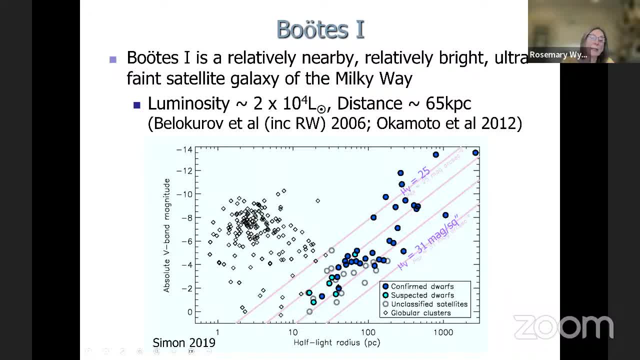 versus half-light radius from Josh Simon's 2019 review. It's actually labeled. notice by these lines are surface brightness. showing you the equivalent surface brightness And these very faint dwarf galaxies is a tiny fraction of the night sky. Again, these are globular clusters and these are candidate galaxies. 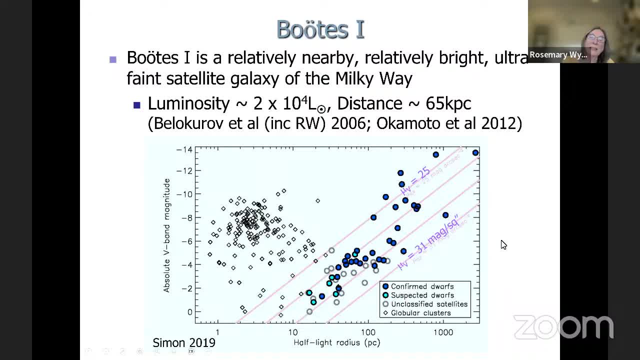 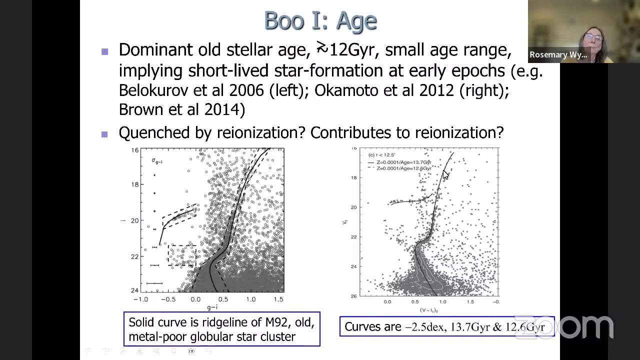 and confirmed and suspected galaxies And we'll discuss how do I know? things are dwarfs. Boötes 1 is this one And the one we just talked about. Reticulum 2 is this one down here, So significantly fainter and a bit lower surface brightness than Boötes 1.. 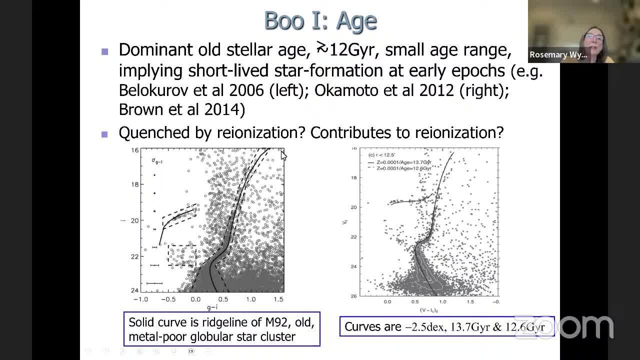 Observationally. Boötes 1, I can get the color magnitude diagram. I can identify a main sequence, a main sequence turn off in a giant branch. I can fit isochrons to this. This is the Okamoto et al's SupremeCam, with Subaru data reaching fainter than the left. 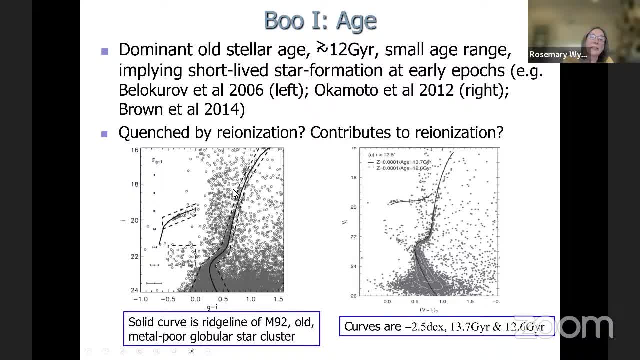 which is CFHT data from Belucoron And the isochrons that fit are metal poor One over 300 times the luminosity, sorry the metallicity of the sun, and very old, fitting very well. The main sequence: turn off giant branch. 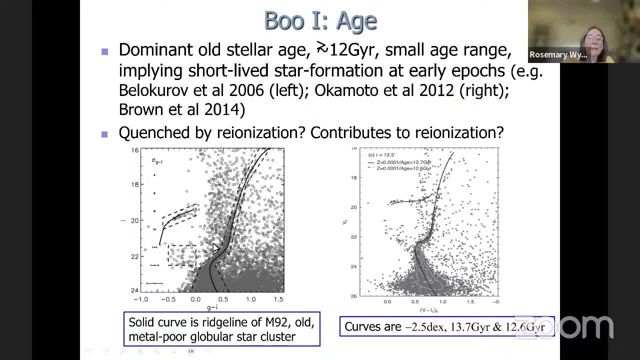 even the horizontal branch On the left here also shows a very good fit. But what's being shown here is the ridge line of an old metal poor globular cluster. So just based on the color magnitude diagram, it just appears the same as a globular cluster. 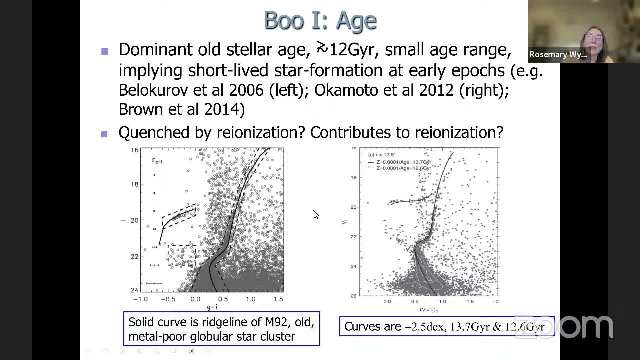 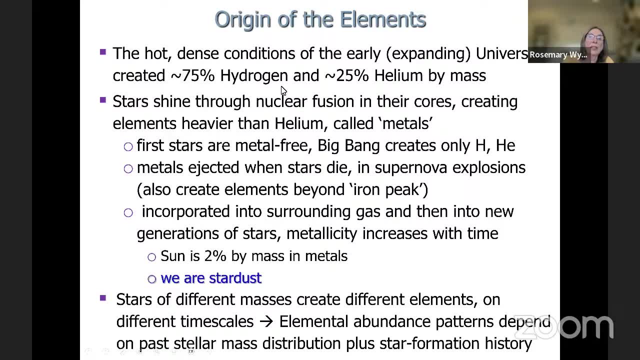 How can we figure out whether it's a galaxy or not? One hint comes from the chemical abundance. So let's just remind ourselves where elements come from. The early universe just gives us basically hydrogen and helium. Everything else comes from stars, And stars create metals in their centers to get new 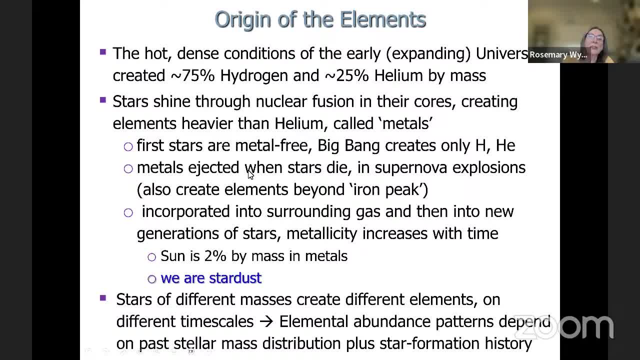 to get new, new, new, new, new, new. to get energy out by fusion, then they radiate that energy. That's why they are shining. When they die they generally explode and that puts back metals so that the next generation to form from gas. 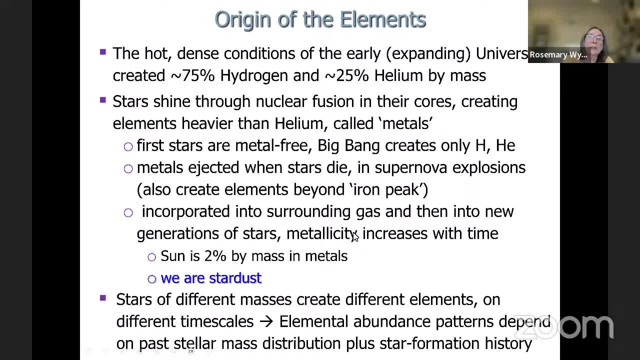 forms from material that's been enriched And we have another cycle of star formation and death, and the metal is today increasing increases with time. The sun is about 2% by mass in metals and, of course, everything of which the earth and us are made of was created in stars. Importantly, stars of different masses create 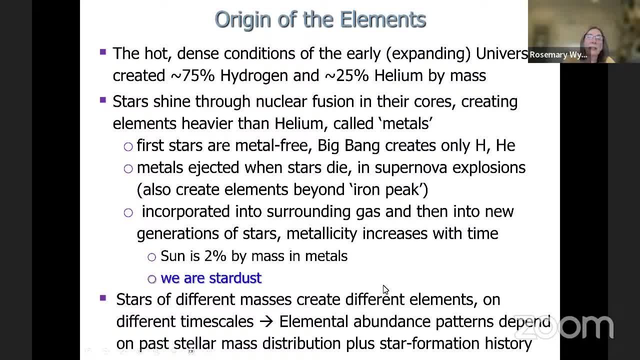 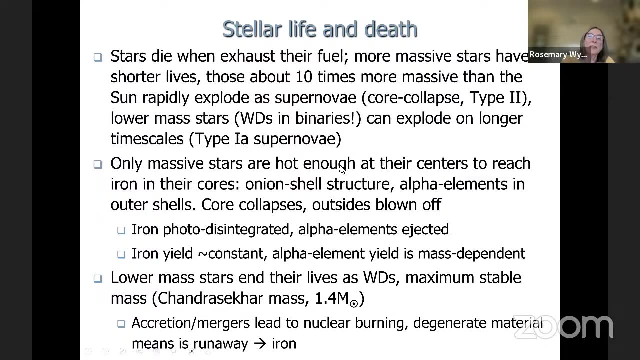 different elements on different time scales, and if I measure elemental abundance patterns of stars in a system, I can get constraints on both the stellar mass distribution and the star formation history. So only massive stars are hot enough to reach iron in their centers. But when they get to iron they can't fuse anymore. 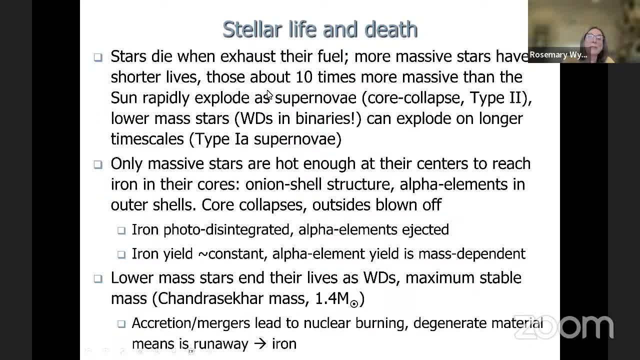 and they explode. These are freeforms, These are irons, These are Scoutron, are massive stars, about 10 times more massive than the sun. they undergo core collapse and in this process, the core, the center, collapses. the outsides are blown off, gets very hot in the center and the 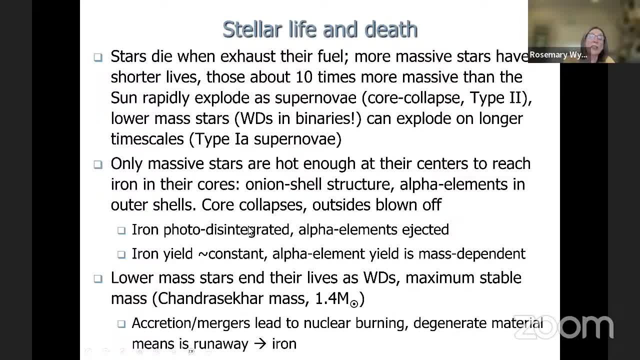 iron that was created during its lifetime actually gets destroyed, but the outer parts which have created so-called alpha elements- those created by successive addition of helium- is ejected. so massive stars produce alpha elements and the iron. a small amount of iron survives and that's approximately constant, independent of the mass of the star, but the alpha element yield is mass. 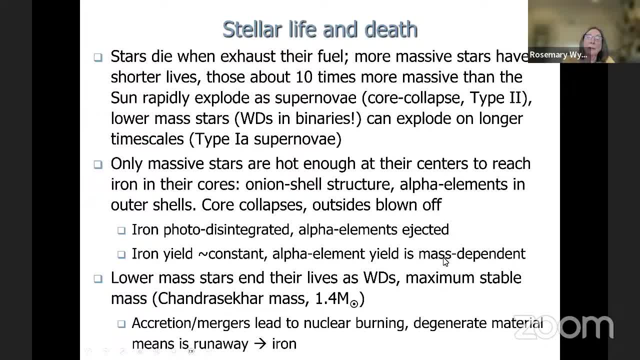 dependent. it is above about 10 times. so between about 10 times the mass of the sun, up to a couple of hundred times the mass of the sun, we get core collapse, supernovae, lower mass stars end their lives as white dwarfs, generally carbon oxygen white dwarfs. these have a maximum solar mass. 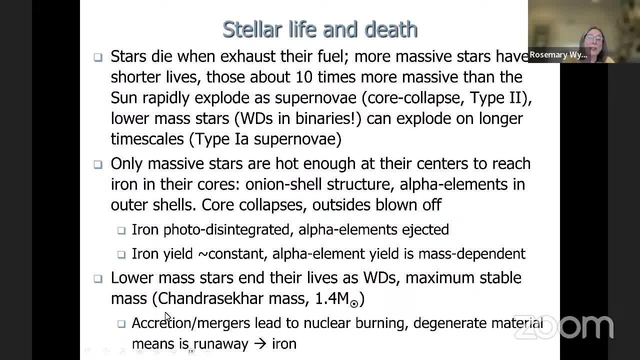 if i get enough accretion or i have mergers of white dwarfs which are degenerate systems- the pressure balancing gravity isn't an ideal gas pressure but is degeneracy of electrons- then i can ignite nuclear burning and if it's degenerate material, 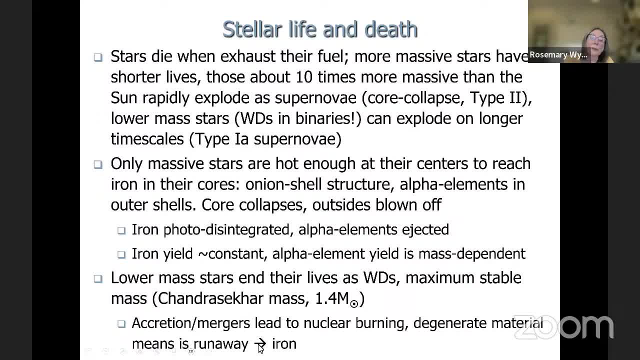 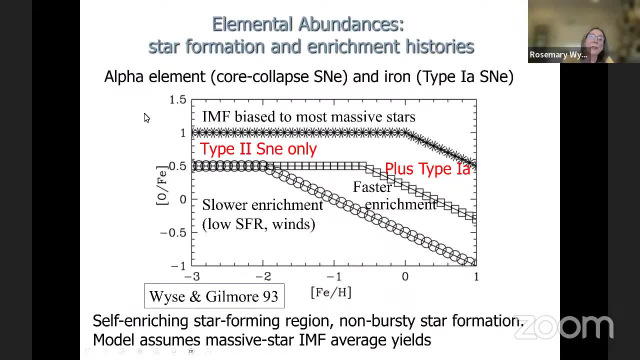 i get a thermonuclear runaway. it goes to statistical equilibrium and i get a lot of iron from white dwarfs exploding as type 1a supernovae. so here's a cartoon of the kind of elemental abundance pattern i would get in a self-enriching star forming region at early times. 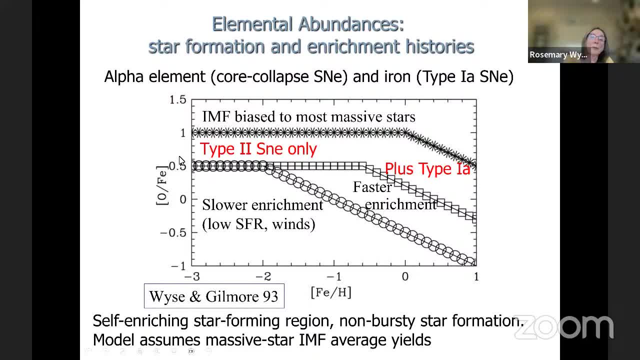 when i have only core collapse, type 2 supernovae. i have a lot of alpha elements, oxygens and alpha element, and i have sufficient alpha elements that it's enriched in alpha to iron about three times that of the sun. after some time i form white dwarfs. i start having white dwarf mergers accretion. 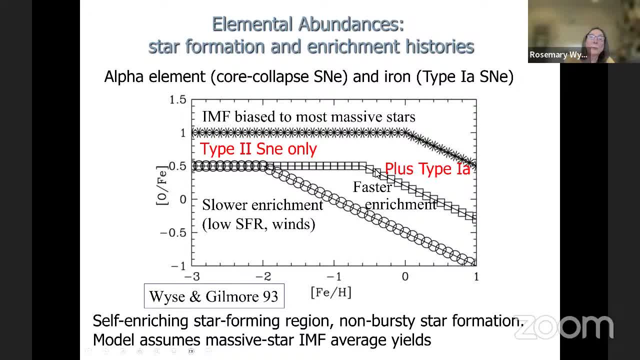 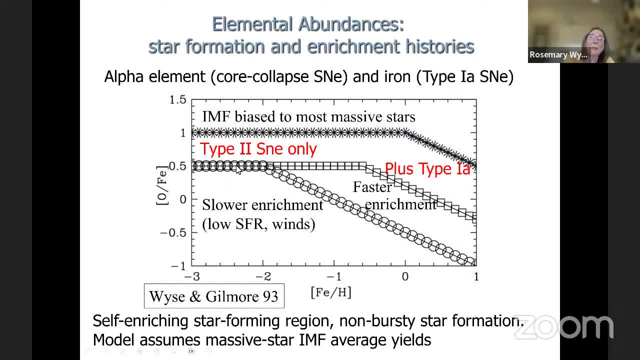 which is against iron, not against time. so the knee is referred to as the knee at which i get iron from type 1a. supernovae depends on the star formation rate. so it's a lot of information, even the imf of the massive stars, because, as i mentioned, you get more alpha elements by mass. 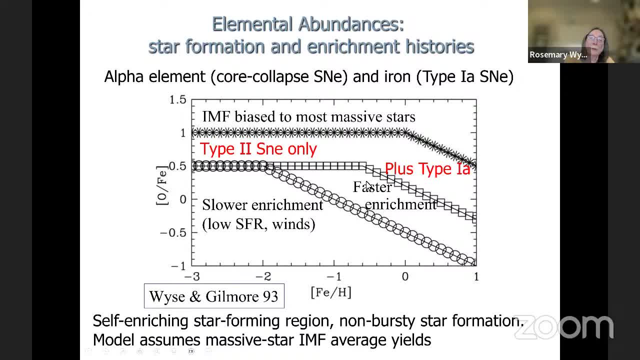 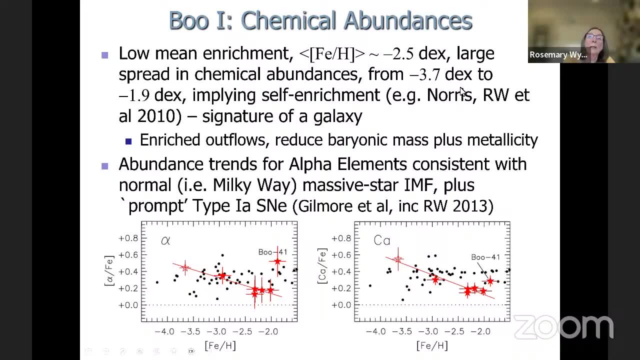 if you have an imf that's biased towards the most massive stars. what do we see in booties one? this is uh earlier work i did with john norris, jerry gilmore- you find very low mean enrichment. the iron abundance is about, indeed, from what fitted the isochrons about one over 300 times. 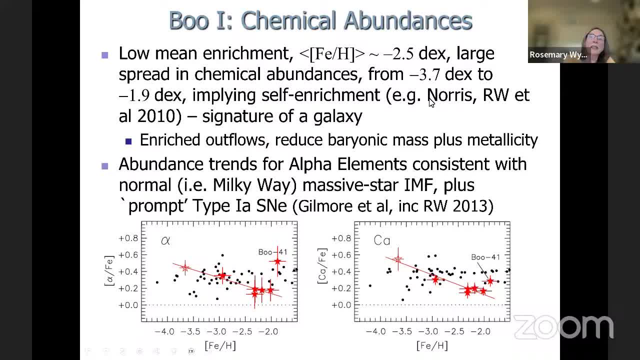 the sun's enrichment. importantly, there's a large spread over two orders of magnitude. that implies some self-enrichment. this is very unlike a globular cluster. this is not a star cluster, it is a galaxy. it has very low mean enrichment, very low baryon content, so very plausibly, its potential well is. 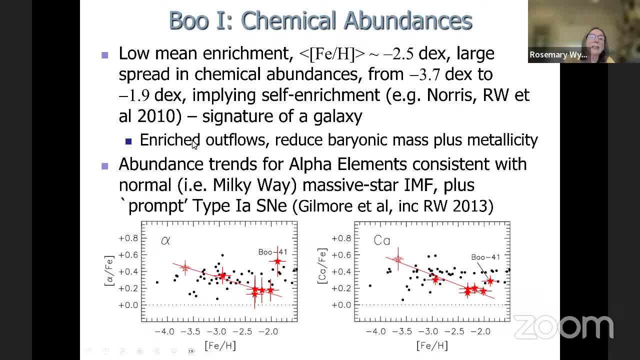 in deepening and it's not a star cluster, it's in deepening and it's in deepening and it's in enough to contain the ejecta from supernovae. that ejecta, a lot of it, blew out of the galaxy. that would reduce its baryon mass plus its metallicity. so here's iron, showing you the small sample for 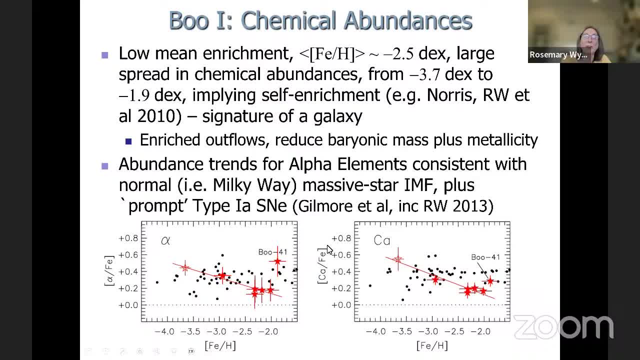 which we have detailed alpha abundances. but you can see here down to the bottom of the cluster which is most powerful of the botanical elements. if we take a look here, there's a very small sample of the baryon mass. that's the absolute largest for the umb in the solar system and you'll see. that the baryon mass is headphones. but the baryon mass is the total number. of course is the number of hours of your year. that is the number of hours that you're going to be going to. that are, of course, that is the number of hours of a year that you're going to use. 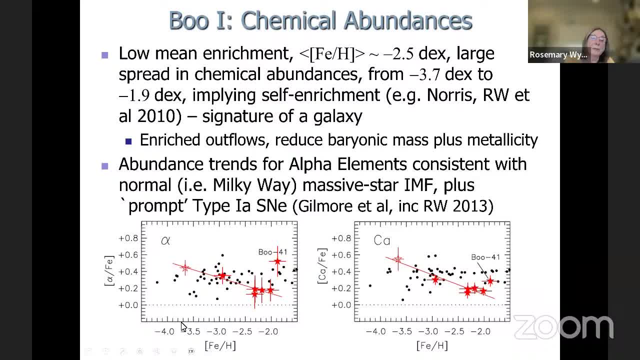 so it's very small. you can reduce it. so we have a some of the four. you know that- to almost minus four, minus 3.7, up to above minus two. There is a trend most seen here in the alpha elements. that's consistent. The value here at the most metal poor star is actually what. 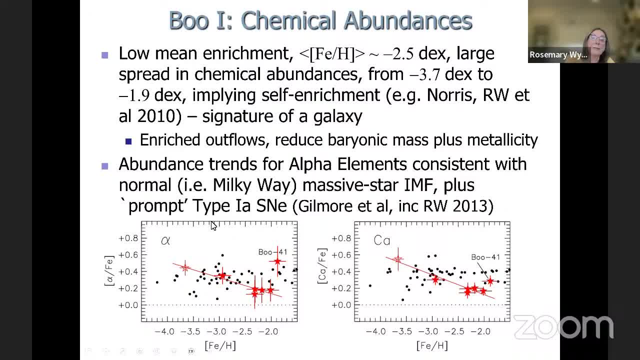 you expect for a normal massive star IMF. This decline is what you would get with type 1a supernovae producing iron. We know there's a very short range in ages, but it could be a billion years From type 1a supernovae. this is if you have a binary of white dwarfs created at the upper. 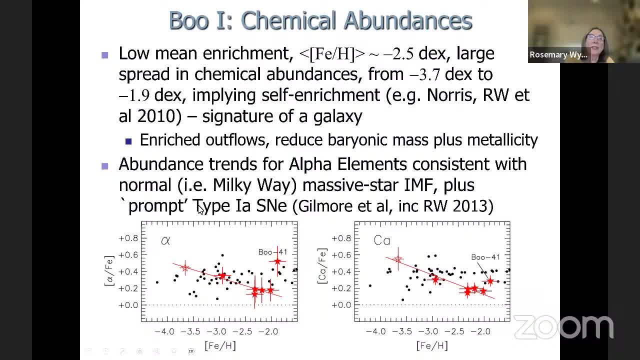 mass of the star. If you have a binary of white dwarfs created at the upper mass of the star, you can get a mass limit of stars to form white dwarfs. You can get type 1a supernovae on a few times 10 to the 8 years That seems to have contributed here. It's self-enriched, It's a. 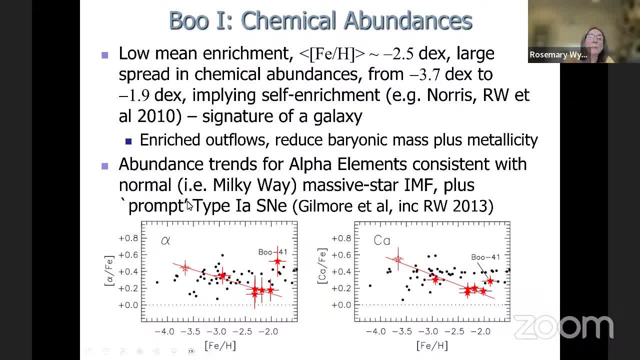 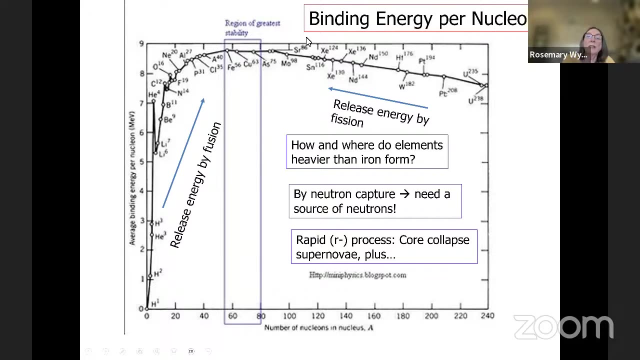 galaxy. It seems to have formed stars with a normal massive star IMF. No change between the mass function at this very early time in a dwarf galaxy and what we see forming stars now in the Milky Way. What about more heavier elements? This is the graph of the binding energy per. 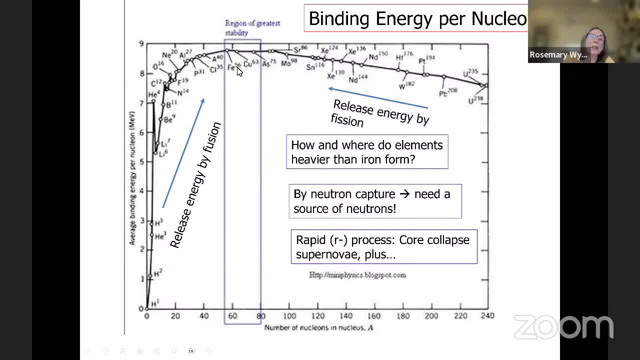 nucleon Stars have released energy by fusing up to the iron peak, but we have elements that are over the iron peak, where you get energy out by fission. We now know that we can create elements beyond the iron peak by actually neutron capture, but then we need a source of neutrons. 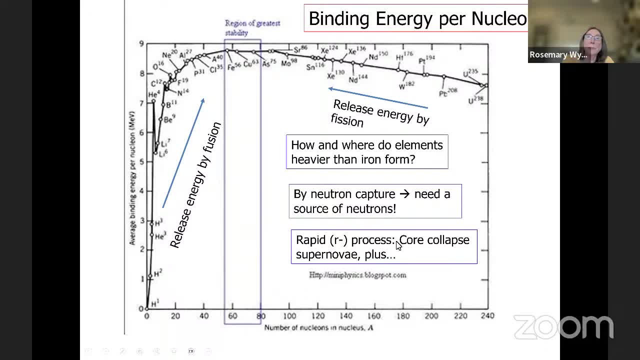 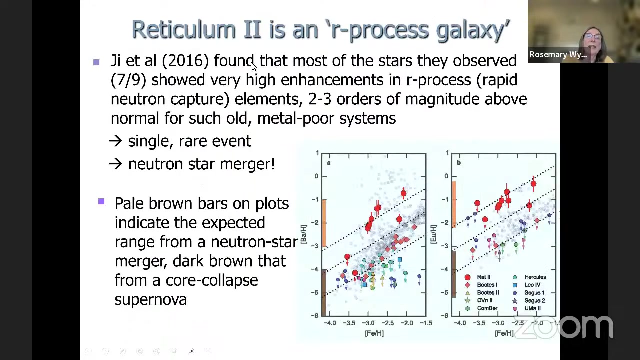 We know that, as I just mentioned, the iron core of a massive star is actually photodisintegrated during core collapse. That gives you a rapid flux of neutrons. It happens very quickly. lots of neutrons. Can we see these in dwarf galaxies? I mentioned reticulum 2.. We'll 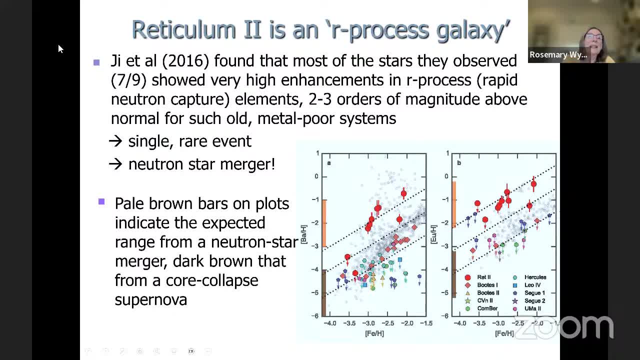 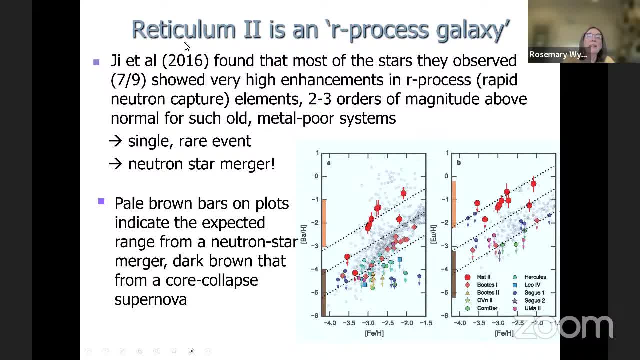 I've been working on for a long time. It's a work that I've been working on for a long time. I think it's very interesting work. LHG et Al got spectra of nine stars in reticulum 2, and found that seven of them. 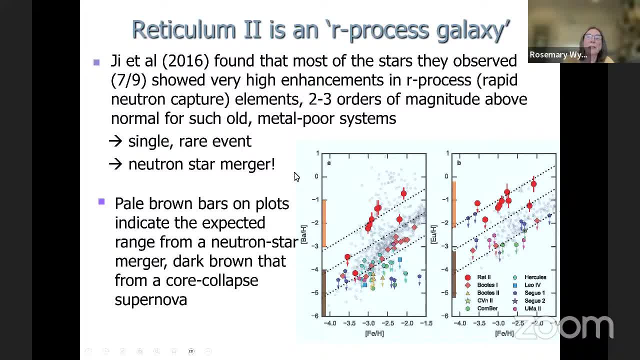 showed very high enhancements in the abundances of barium and europium elements over the iron peak that have a large contribution to their creation through the iron core process. rapid neutron capture: It's rapid with respect to beta decay, So you can so. 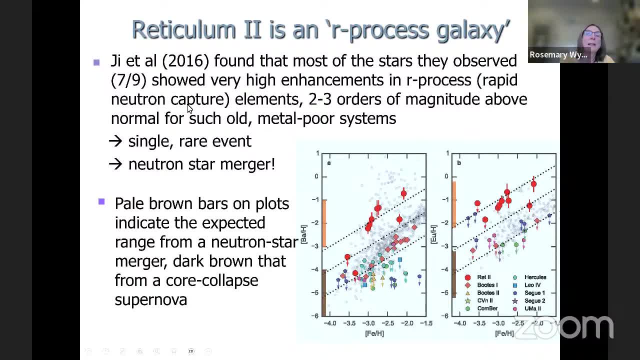 these are unstable nuclei you form and which then decay, And the R process is when you add many neutrons before you have beta decay. Most ultra faint dwarf galaxies don't show this. I mentioned, or at least I should have mentioned, one thing that's important for 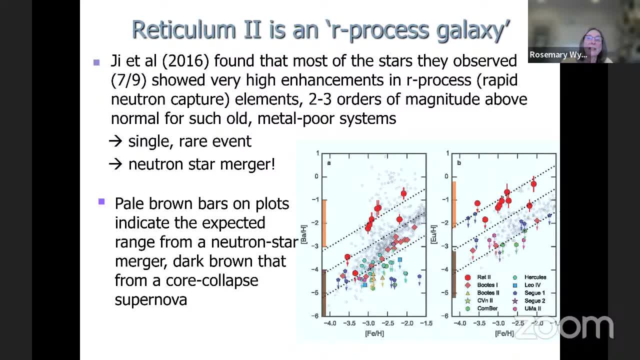 studying these dwarf galaxies? is that plausibly all the stars formed in the system? We think the halo of our galaxy has formed from disrupted systems And, depending on when those disrupted systems were assimilated into the Milky Way, they get very spread out. 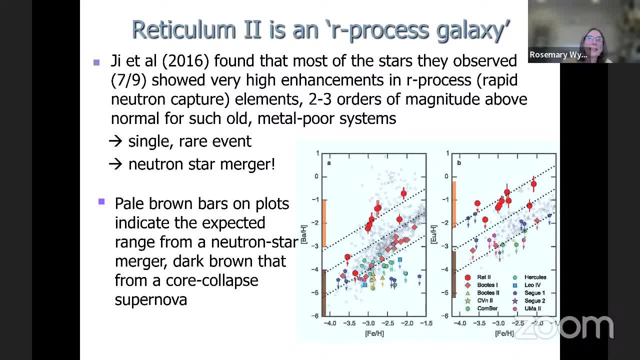 And it's very hard to identify exactly which star formed in which system. If we have an intact dwarf, it's really quite plausible that all the stars formed together and were enriched in the same event. So this is a plot of barium to hydrogen versus iron europium. 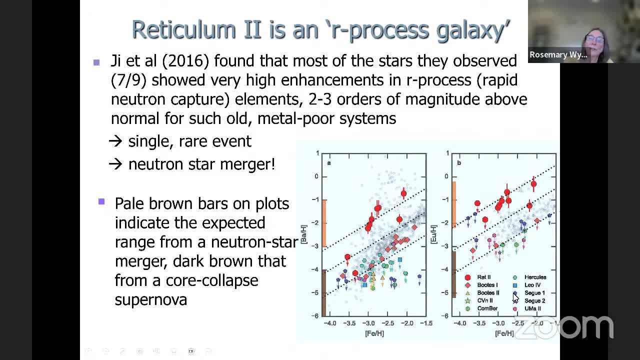 to hydrogen versus iron for a whole load of ultra faint dwarfs. Most of them lie below the red points, which is reticulum two. The pale brown bars here on the y-axis is the expected range of barium and europium you get from a single rare event: a neutron star merger. 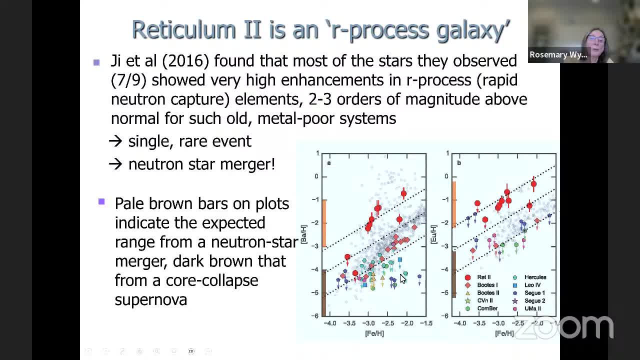 Dark brown at lower values is what you would get from core collapse supernovae, And that is why they seem to form like white dwarf stars. By the way, I would also like to point out that this is part of the numerical analysis. on the gray bar, in the yellow bar, The white bars on the white line areWaiting for the 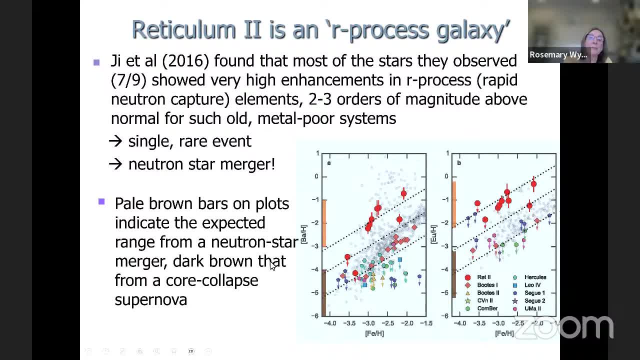 sun to rise, which means that there is no future until the sun is rising, And we often see the same thing with the stars. This is a clear example of how they are actually formed, and the way they represent the stars is very, very interesting. So I don't know if you've been interested in our show, but now 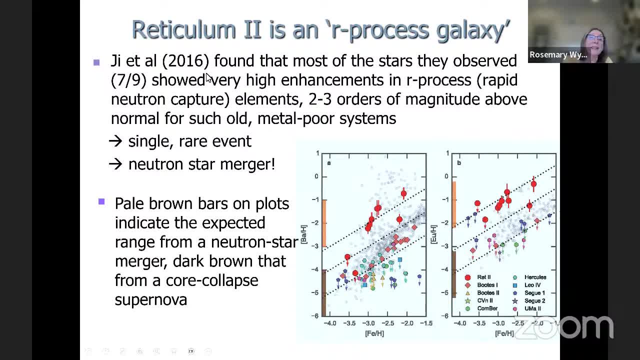 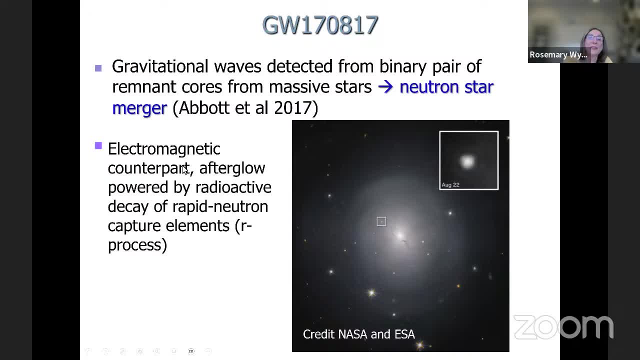 but we hadn't seen any. but then in 2017, we actually did detect a neutron star merger. not only that, but this neutron star merger, GW170817, was localized on the sky and there was an electromagnetic counterpart. you can see the brightening here over several days. 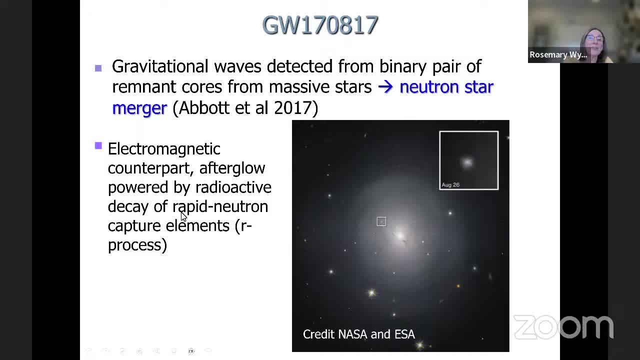 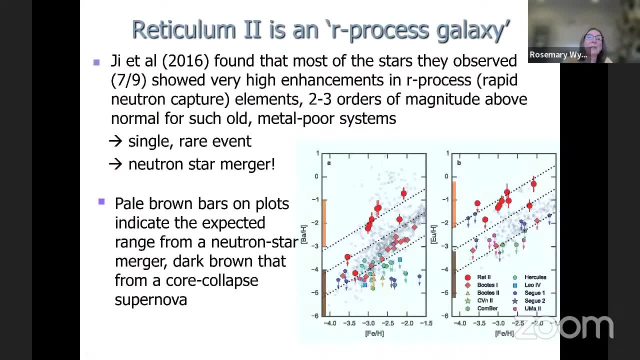 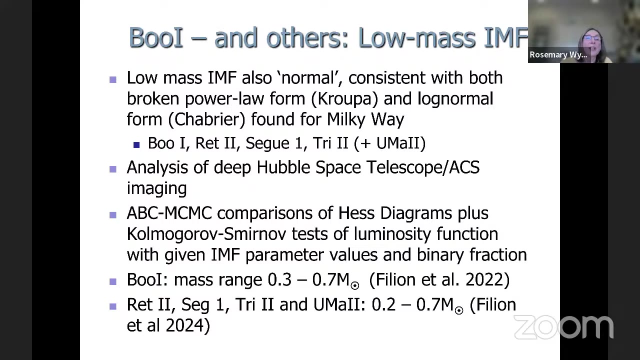 plausibly powered by the radioactive decay of the r-process element. so everything hanging together. but Alex G et al found the signature in the elemental abundances first. I will speed up a bit. so, returning to booties one, we have the chemical abundances of massive stars being consistent. 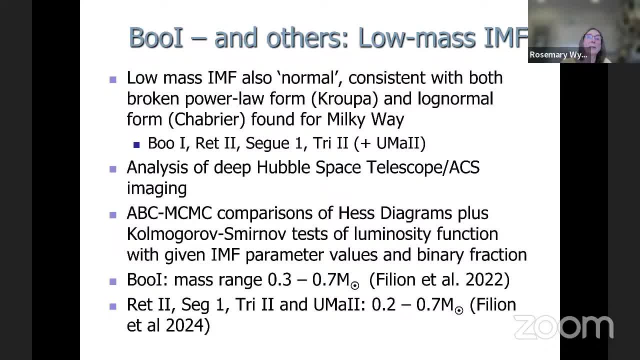 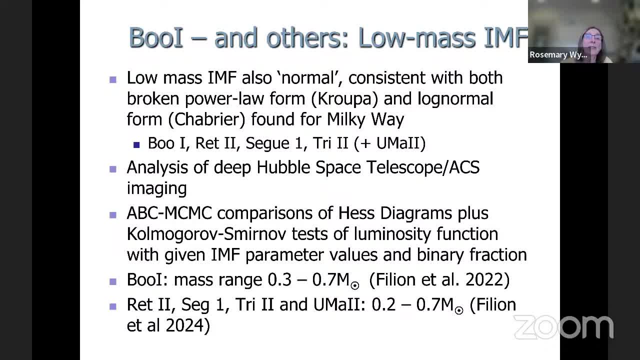 to the halal came from many different points of the star. that might be relatively simple, and it's in the monochromatic field and it's also verywangstonstable. so this new molecular form descaling from a monochromatic field of the star, which is the same as what? we see in the infrared field of light, as we see in the andromeda, and it's the same as the'the', the'the', the'phelion', the'phelion' that's coming out of the limestone. so we've got a very large group of stars that've been lie in the limestone and have got very much of the light on its surface and there are very large amounts of the light on the planet's surface. there's a very big number of stars that's coming out of the sky. that's coming 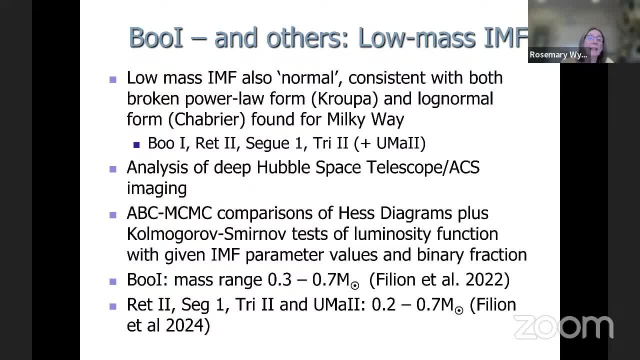 from zero. so we can see that in this particular example we have a very big and very deep scope imaging, doing various analyses, including ABCMCMC, that's approximate Bayesian calculation with Monte Carlo Markov chain or by comparisons of the Hess diagram, the binned color magnitude. 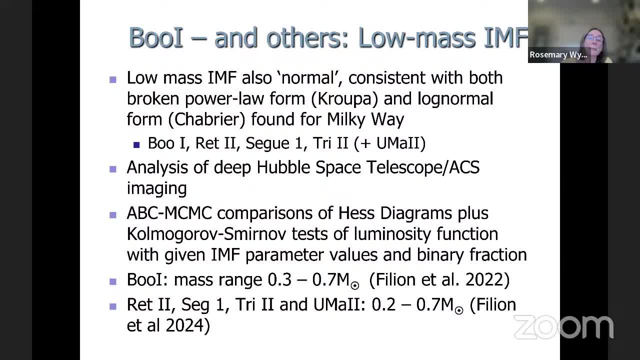 diagram plus Kolmogorov-Smirnov tests of the luminosity function against given IMF parameter values and binary fraction. to figure out what is the single star mass function in these ultra faint dwarf galaxies, It's very important to have comparable ranges. 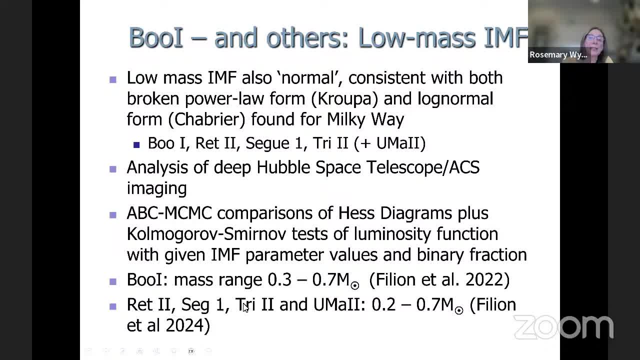 It's very important to have comparable ranges of masses in the systems you're studying, to be able to do an intercomparison and also to go faint enough that you have some constraint on where a turnover might be in the mass function. What we've found is that in all these systems, the IMF is consistent with the power law form. 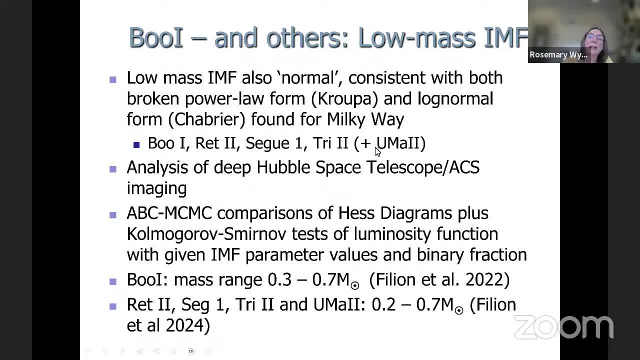 of the IMF, The multivariate. I've put Ursa Major2 in brackets here because it's only consistent with the broken power law form. There's a slight inconsistency with the log normal form. If you read the paper just about to come out, you'll see that the Ursa Major2 field has. 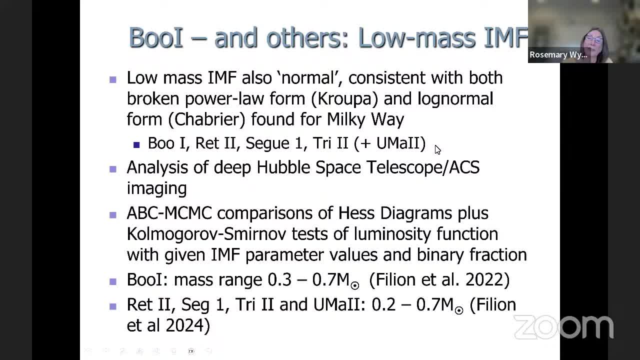 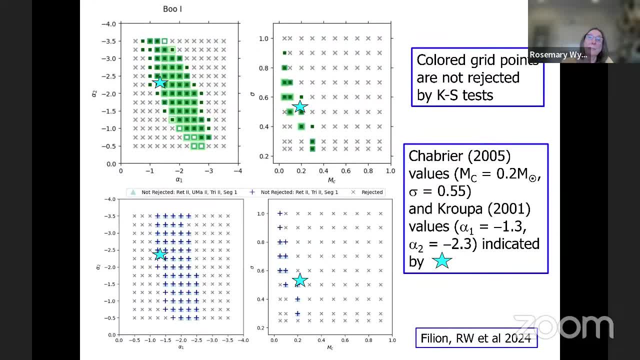 known intermediate redshift galaxy clusters, so we're not 100 percent confident. we removed them all. it's just a plot. from the 2024 paper booties, one was analyzed separately in a 2022 paper. we re-analyzed it in the same way as the four other dwarf ultra faint dwarfs. 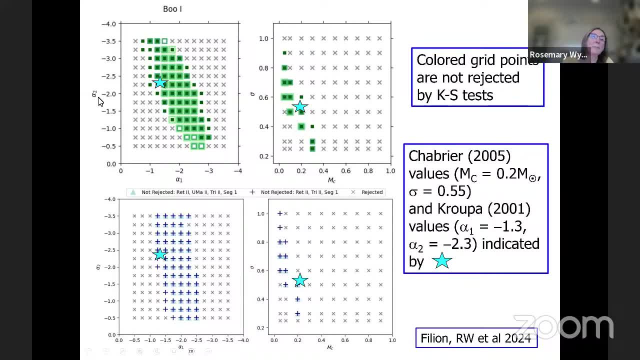 these are grid points in imf parameters, for instance the two slopes of the broken power law or the turnover mass and the width of the log normal. the colored points here are imf parameter values that are not rejected and the stars are the milky way. upper is just for booties one. 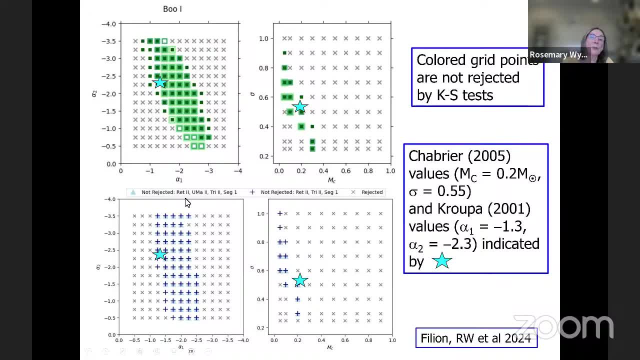 low combines all the four dwarfs, reticulum 2, ursa major 2, triangulum 2 and segue 1 together for the overlap that they're all consistent with this particular combination of power loss slopes or log normal. this does not include ursa major 2 here. 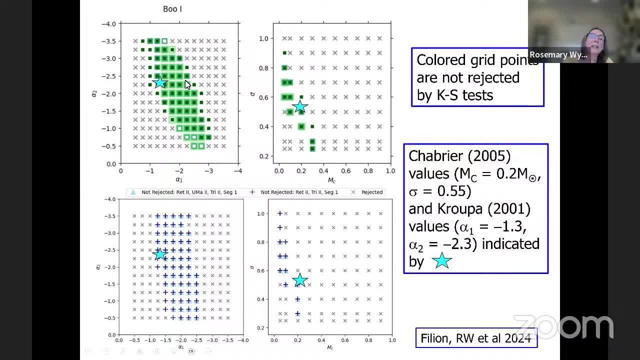 and what you see is that the colored points are fine and they are consistent with the local values. the local values are, as to be said, at the edge of what's not possible to reject, but are still consistent with this set of dwarf galaxies. So we have a normal. 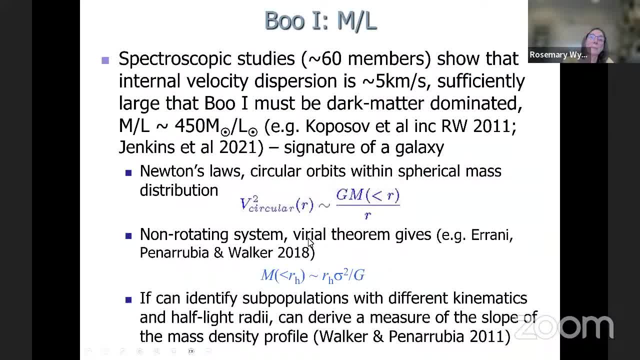 massive star IMF and a normal low mass IMF. What else Just in the last few minutes? what else makes a galaxy? Well, it has to have dark matter. We now have enough spectroscopic studies of Boötes 1 to know that the stars don't provide enough gravity. 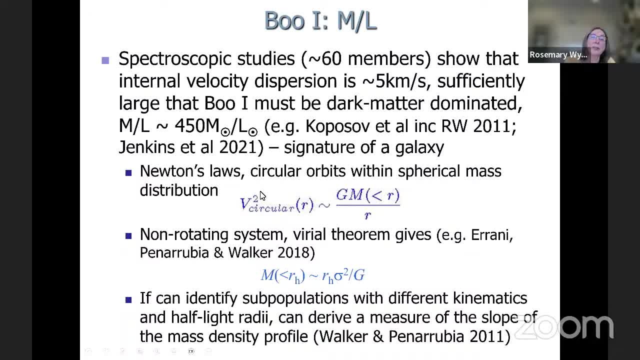 to keep it bound must be dark matter dominated. Just remind you that you get enclosed mass by having some measure of the range of velocities with which stars are moving. These are non-rotating systems. There's a mass estimator within the half light radius. that's of order. 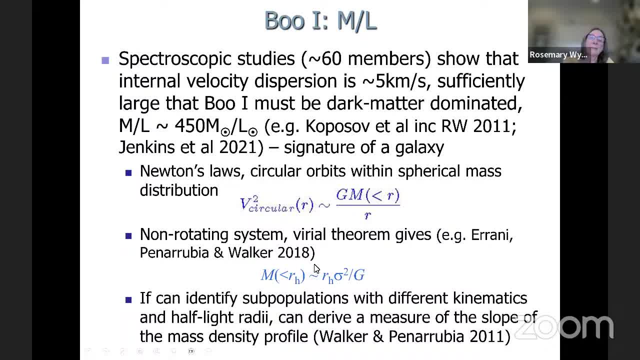 given by a factor constant, a few half light radius velocity dispersion squared over g. If you can identify subpopulation, say by their kinematics and half light radii, you could apply this mass estimator using two different half light radii, two different characteristic velocity dispersions. 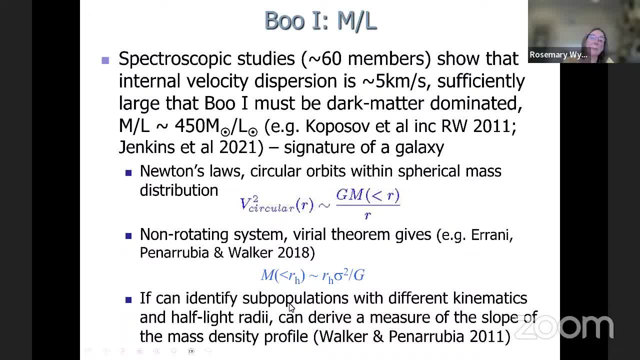 The subpopulations are in equilibrium in the same potential. well, but I can get a handle on the enclosed mass at two points and I can get a measure of the slope of the mass. I can get a measure of the slope of the mass density profile. 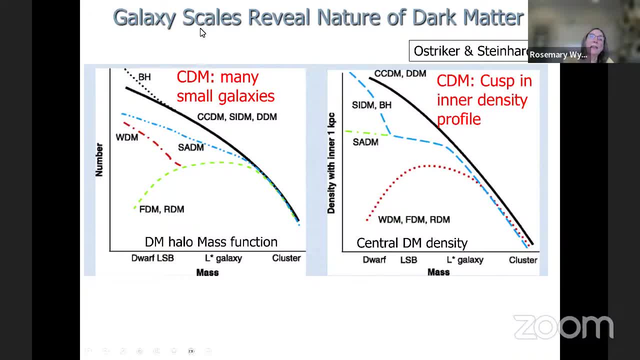 Why is this important? Just to remind you again, it's galaxy scales where you start to see the nature of dark matter On very large scales, clusters of galaxies, the microwave background, gravity is dominating and all dark matter. There's many different types of dark matter shown here. 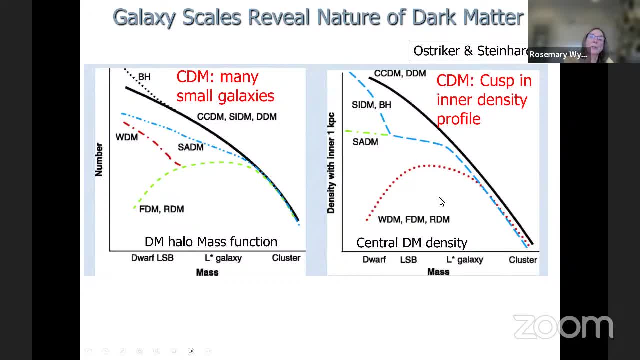 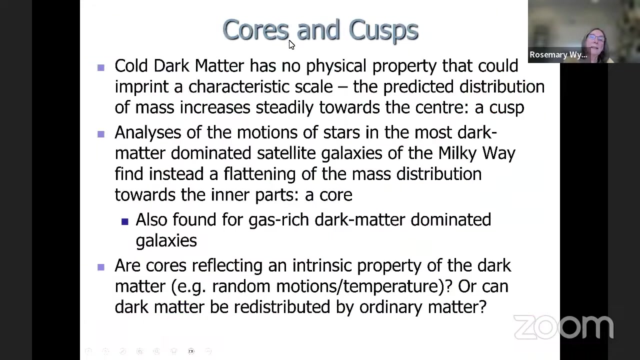 A plot from Ostraikon and Steinhardt in 2001.. At large scales, all the different dark matters agree. It's only on individual galaxies, in particular dwarfs, you see the biggest divergence in predictions of properties such as inner density profiles. 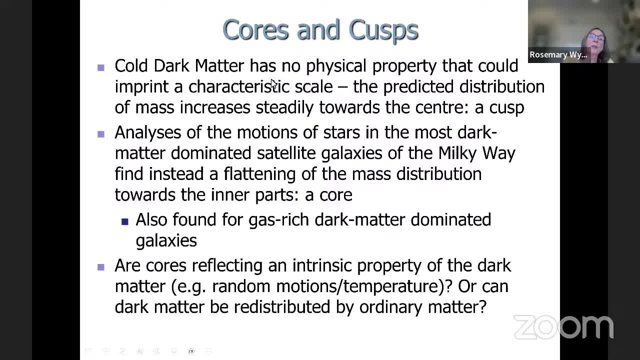 If I have a few more minutes, Cores and cusps. indeed is a very important tension between the predictions of cold dark matter. Cold dark matter: no physical scale that could imprint, sorry, no physical property that could imprint a characteristic scale. 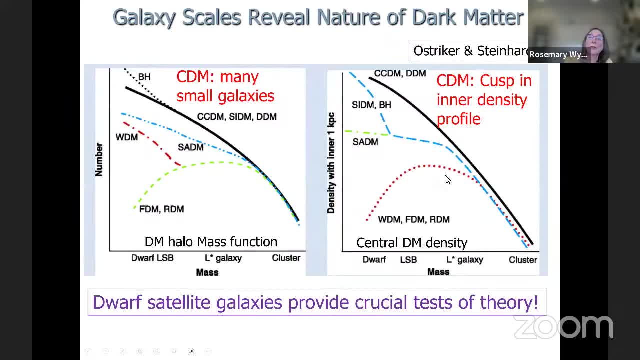 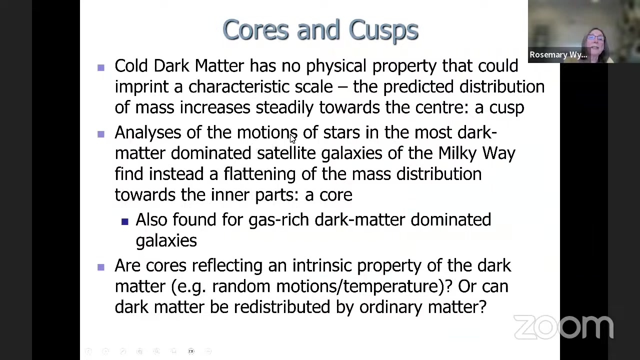 That means the predicted density distribution for cold, collisionless dark matter just steadily increases. There's a power law towards the center, No scale, like you can see here for fuzzy dark matter. So they predict a cusp. However, if you analyze the motions of stars in the most straightforward way, 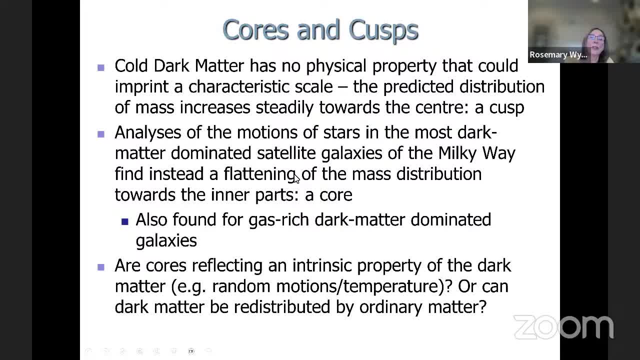 you get a core in both dwarf spheroidal galaxies and gas rich dwarf galaxies. A question is: is this core the intrinsic property of the dark matter, such that streaming motions, Or can you redistribute dark matter such that it starts with a cusp? 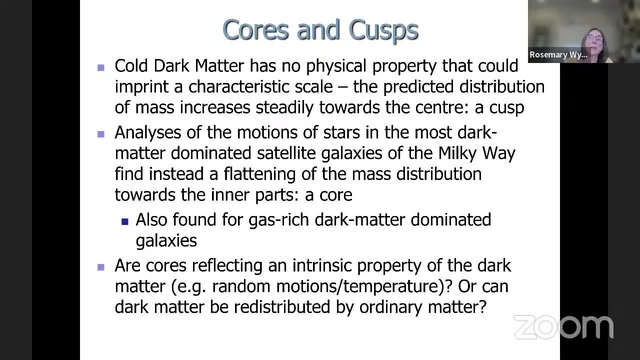 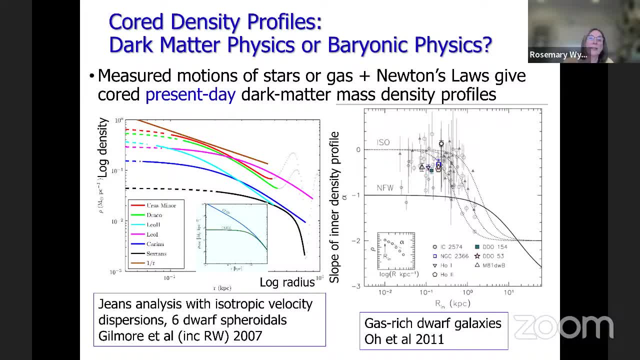 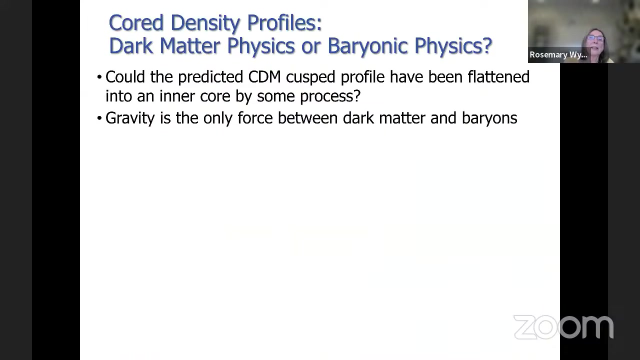 it is cold dark matter. somehow that cusp gets erased. These are just plots showing you that both gas poor and gas rich galaxies have cored present day dark matter density profiles. But the issue is: has that been created by the gravitational interaction between dark matter and baryonic matter? 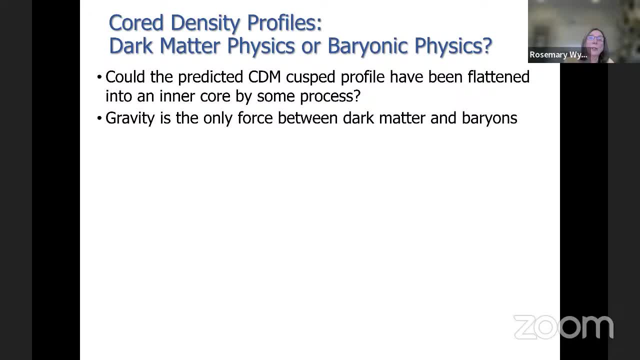 So could gravity? could this work? that a cusp profile be flattened? And the answer is yes, it could. If I have rapid injection of energy and momentum from short-lived massive stars, I can create a new equilibrium state which has less dense inner regions. 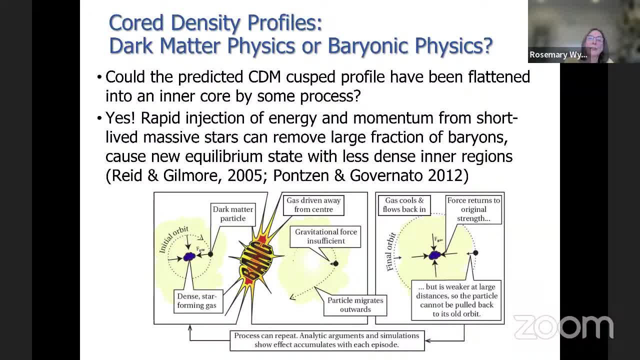 Very influential paper, Ponzin and Govornatu. little cartoon here you can look at, showing how, if I have a lot of baryons in gas at the center, I can form stars. I can change the gravitational potential sufficiently that the equilibrium distribution puffs up. 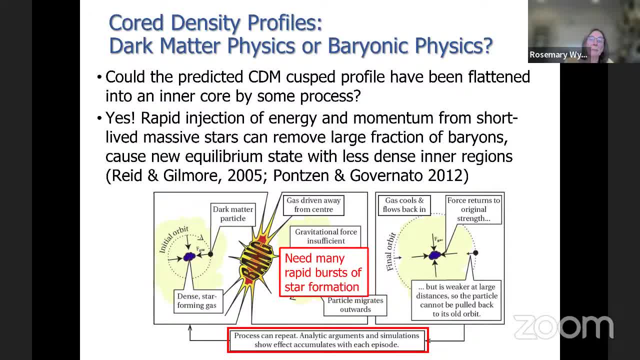 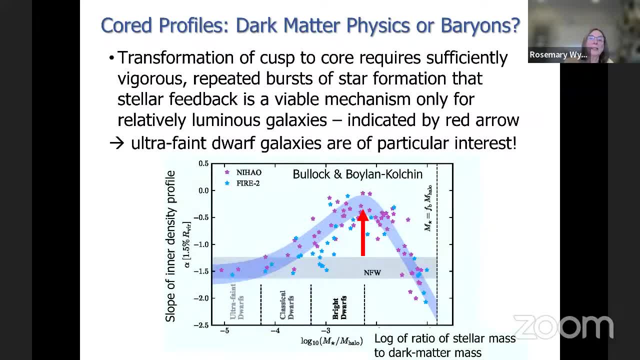 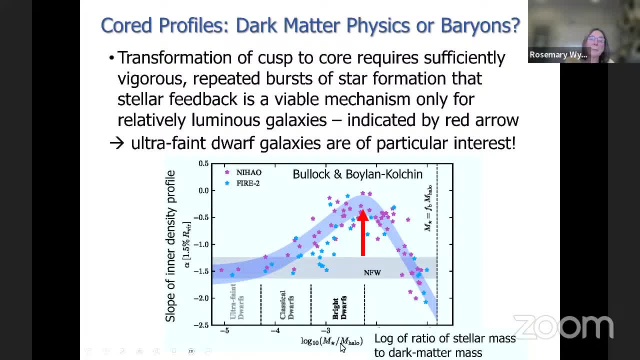 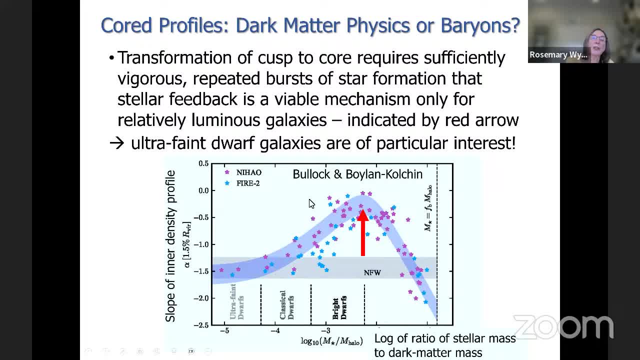 I can change it to be close to constant density through repeated bursts of star formation. provided this is a plot from Bullock and Bull and Koshin, this does work. This is seeing in simulation. But only if I have enough baryons, enough star formation doesn't work. 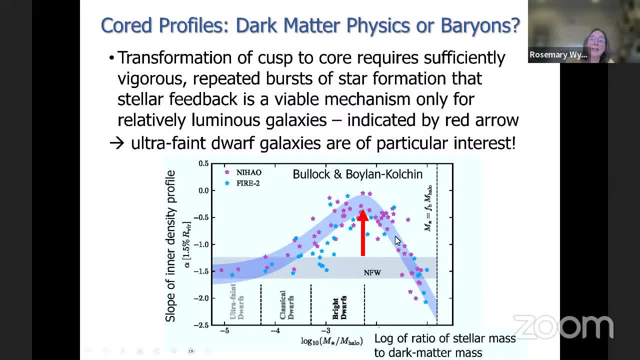 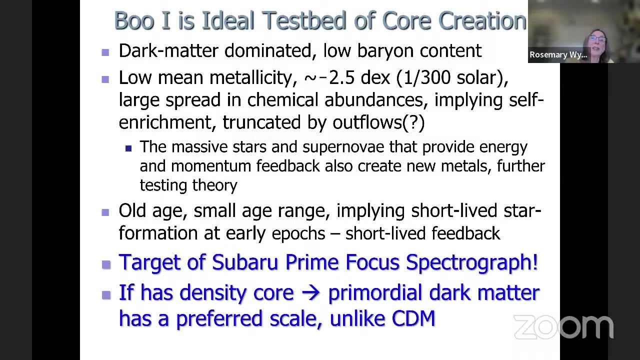 There's no difference between the present day mass function indicated by the purple and the primordial cold dark matter density profile for ultra faint dwarfs. So Booty's one having lots of dark matter But very low baryon content. small spread in star formation history, small spread in ages is an ideal testbed of this idea. 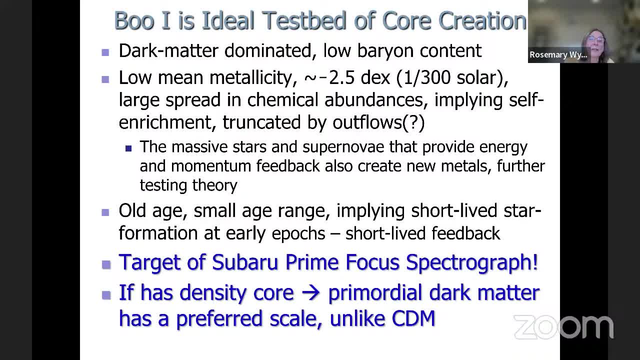 And it's a target of the Galactic Archaeology Survey. with the Subaru Prime Focus spectrograph We want to determine the mass profile, probably by finding subpopulations constraining the interior mass at different radii. If it has a core, then that means dark matter has a preferred scale. 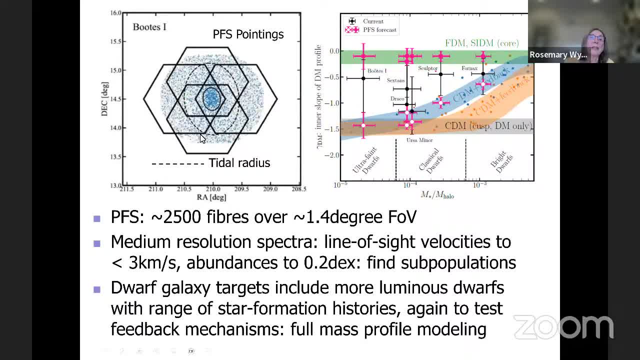 Just to run through this, here's the PFS pointings for Boötes 1.. This is the half-light radius on the sky And nominal tidal radius. We're going to cover the whole face of it with many pointings, each with 2,500 fibers. 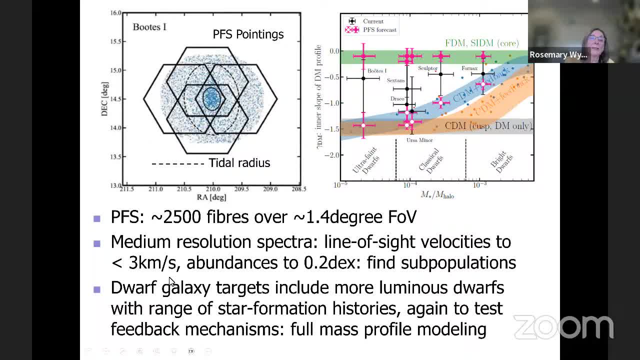 Medium resolution spectra will get good line-of-sight velocities, good abundances, fine subpopulations. Here's a different version of that plot, showing the forecast for the error bars that we'll get for Boötes 1, where we 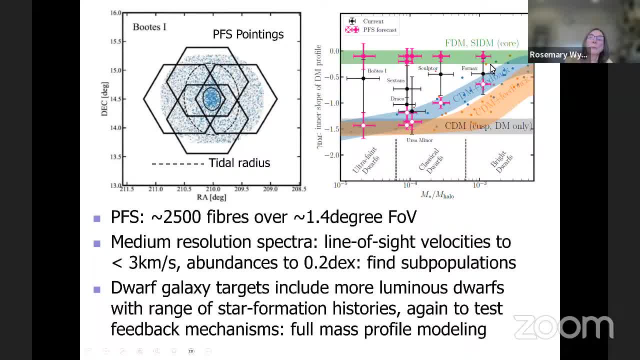 Find subpopulations And for the other, more luminous galaxies. of our sample, these are selected to have a range of star formation histories So we'll be able to distinguish cold dark matter, predictions from baryon changing the profile and also other more exotic forms of dark matter. 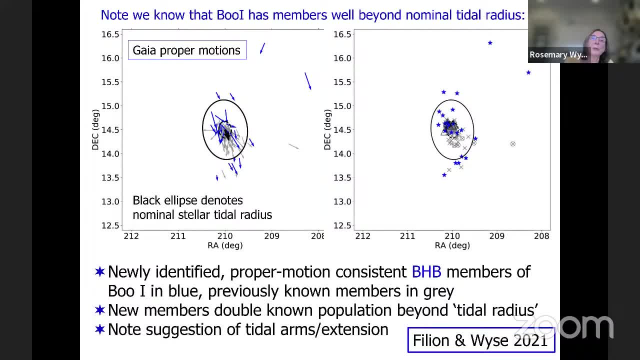 So we actually know that Boötes 1 does have members. You might say: why are you spending time to go out there Again? Carrier-Fillion has identified blue horizontal branch stars that are Gaia. proper motion apparent magnitude consistent with members. 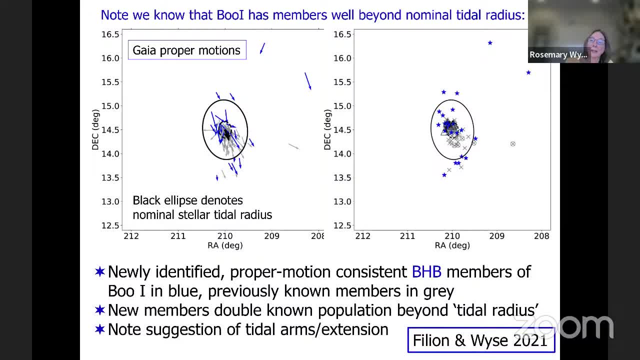 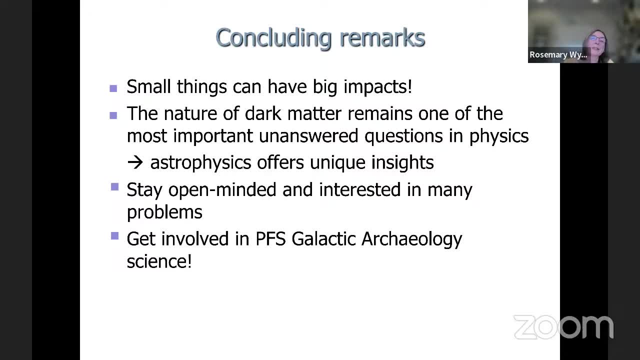 So we're really going to map the full extent of the dark matter. So let me just conclude Concluding remarks. I hope I've convinced you that small things can have big impacts. We can figure out the IMF at high redshift. We can perhaps figure out the nature of dark matter. 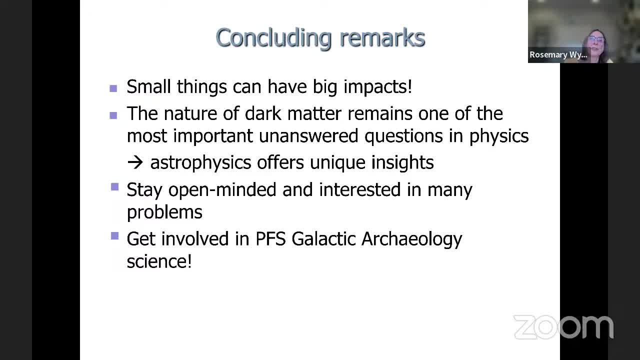 And that's one of the most important unanswered questions. We get unique insights from astrophysics, very complimentary to direct searches To the graduate students and undergraduates. stay open-minded during your career, stay interested in many problems and perhaps get involved in PFF- galactic archaeology. 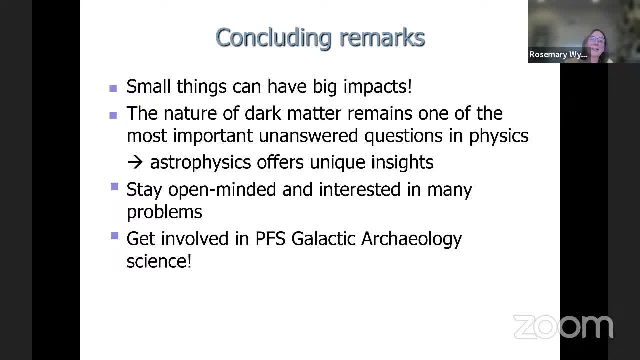 science. Send me an email if you'd like to understand more about that, Thank you. Thank you, Rosie. Do we have questions from the audience? first I have a question. Can you come closer to the camera? Hi, Rosie, Hi. 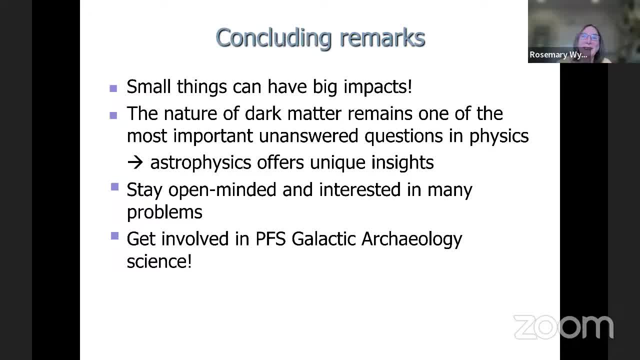 Thais is here. Oh, hello, Hi, Hello, Thais. Yeah Bye. I have a question. I have not such related question to dark matter, but I wonder if these dwarf galaxies have to do with the very in the beginning of the universe, these dwarf galaxies that are being 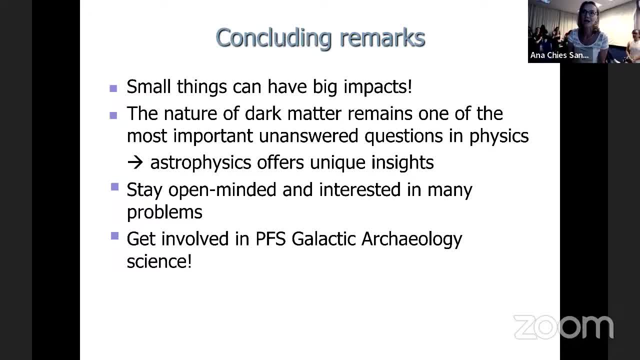 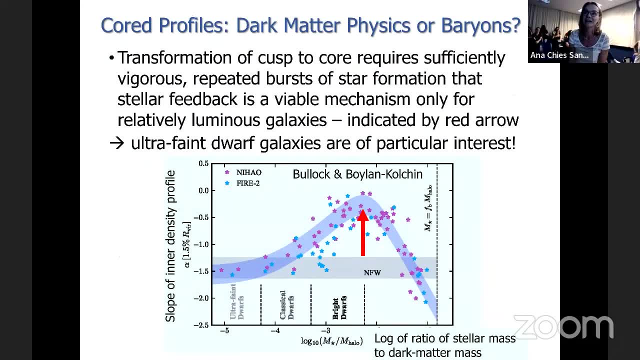 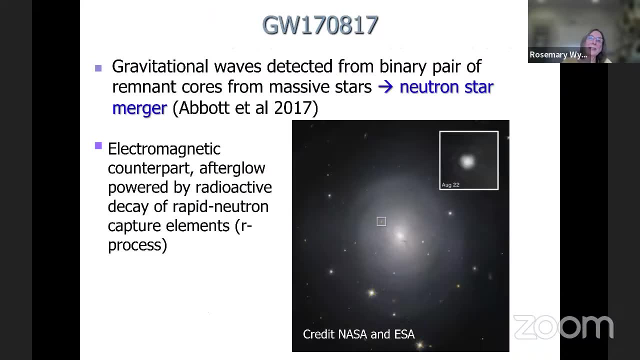 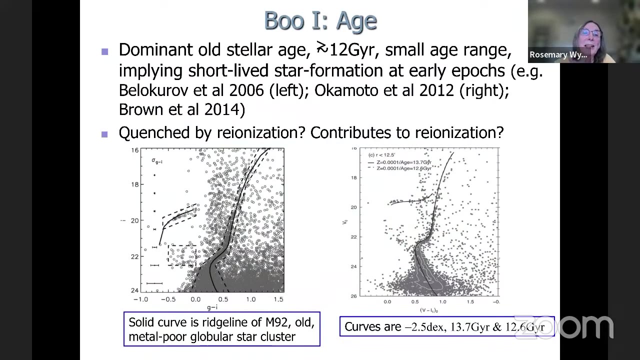 argued to be the realization sources of the universe Could be these dwarf galaxies that you are studying now, those dwarf galaxies that were realized in the universe in the beginning of the universe. Yes, So let me just go back to the age distribution Back here. Yes, So it's very interesting to 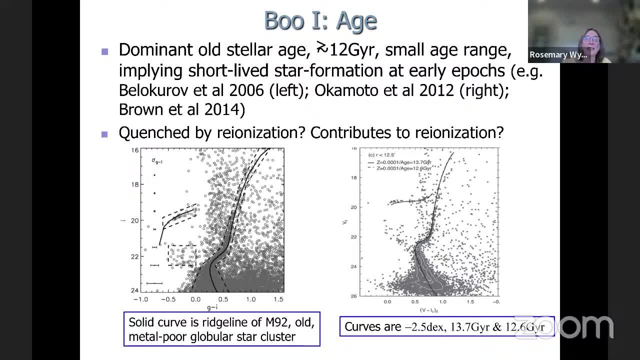 try and really pin down the ages of the stars in these galaxies. As you're probably aware, old metal, poor stars, more or less, are the stars that this galaxy is in, And so, in the past, the stars that have been found in this galaxy have been found in the stars that are 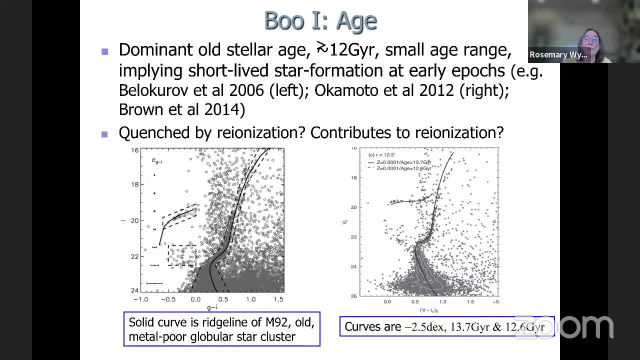 in the stars that are in the galaxies. Yes, Yes, Yes, Yes, Yes, less look the same, independent of whether they're even 11 billion years or even 13.6 billion years. so we would like to know: are they quenched by? you know? did they form most of their stars before? 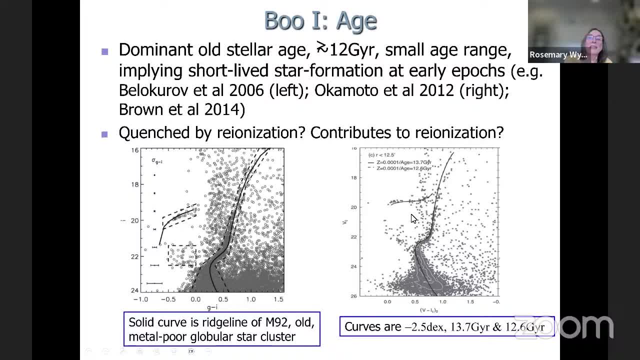 reionization. did they continue forming stars through reionization? are there enough of them and do they have enough photon leakage that they could contribute to reionization? I suspect that it's the more luminous, not the ultra faint, the more luminous galaxies. that would be the one. 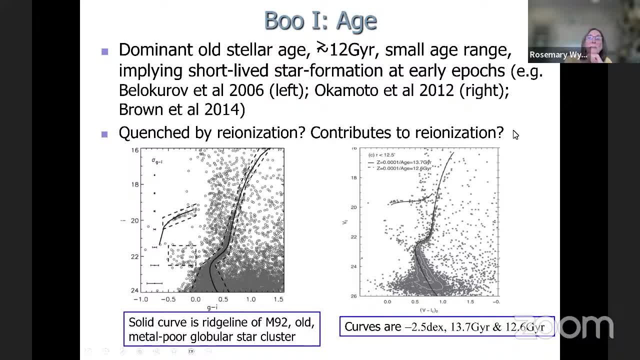 ones that contribute to reionization, but these are certainly of an age to be forming stars around that time, and it's very interesting to try and figure out what happens to star formation through reionization. Thank you, Yeah, Yeah, Hello, my name is Mirjani. 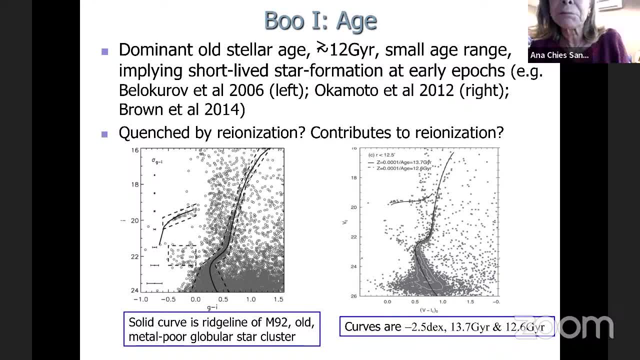 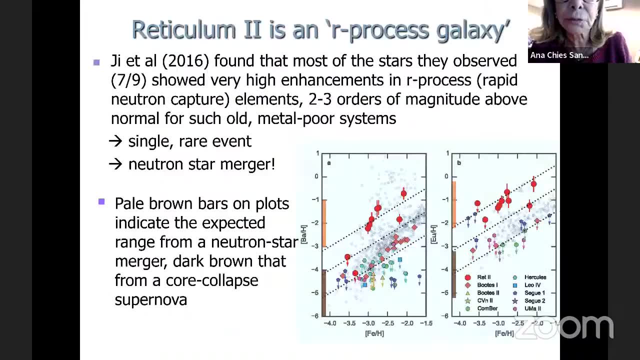 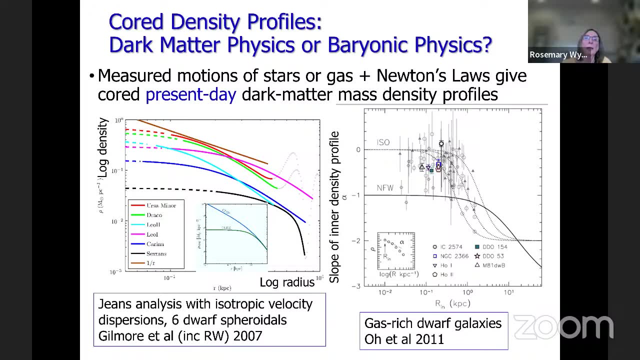 My question is about the distribution of the dark matter in these galaxies. Does it follow the Navarro profile or have a different profile? So the systems that we have in the galaxy, the galaxies that we have in the galaxy, they are the ones in which we have good measurements of the velocity dispersion as a function of 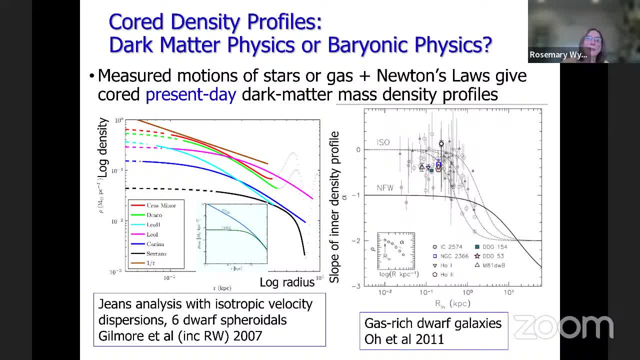 position are shown here. Now, when we are only measuring one component of the space velocity, which is the line of velocity, there is an ambiguity in how you analyze the data. So it is always possible to find a version of the Navarro-Frenken-White that can fit. 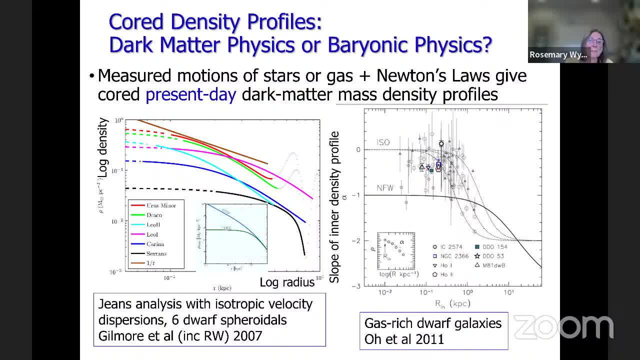 any one particular dwarf galaxy, But what we've shown here is the entire galaxy. So it is always possible to find a version of the Navarro-Frenken-White that can fit any one particular dwarf galaxy. So it is always possible to find a version of the Navarro-Frenken-White that can fit any. 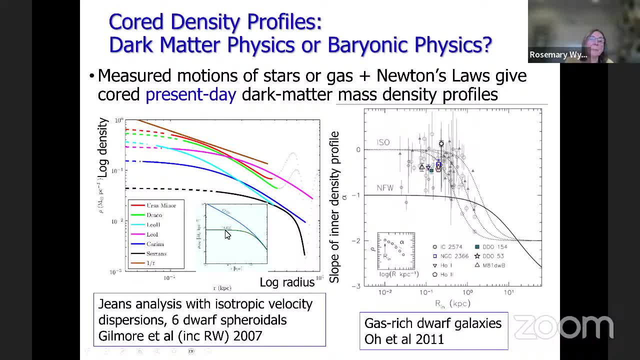 one particular dwarf galaxy. But what we have shown here is the analysis of the spatial distribution of the starlight and the velocity dispersion, the line of sight velocity dispersion as a function of radius For six dwarf spheroidals with a range of star formation histories. but we have assumed 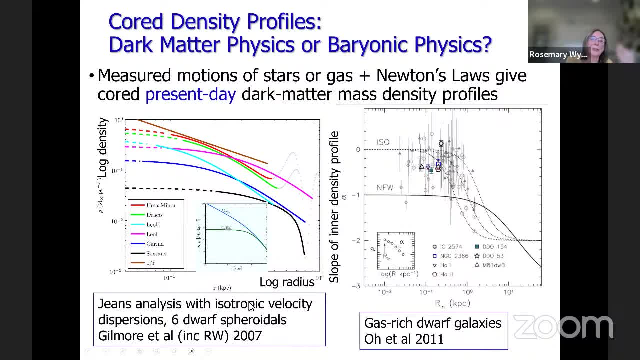 an isotropic velocity dispersion. So it is almost impossible to find a version of the Navarro-Frenken-White that can fit. and we find that they do not fit the nfw profile. there is a turnover as opposed to the cusp that is predicted for nfw. this work was criticized because we assumed isotropic. and there's what's. 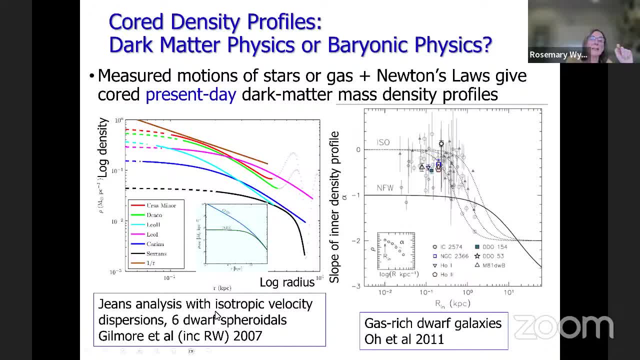 referred to as an anisotropy mass degeneracy, in that in the genes equations, the equations that we used in this analysis, you can have a different mass profile if you allow the anisotropy to change as a function of radius, or just be different from zero. but our argument 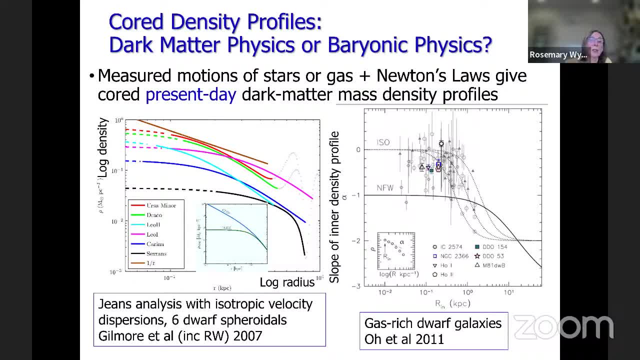 is that these are very different dwarfs. if you allow the anisotropy to be non-zero, then you would expect it to be different for the different systems. they have different star formation histories, different orbits about the milky way, different total luminosities. you would not a priori expect to get the same. 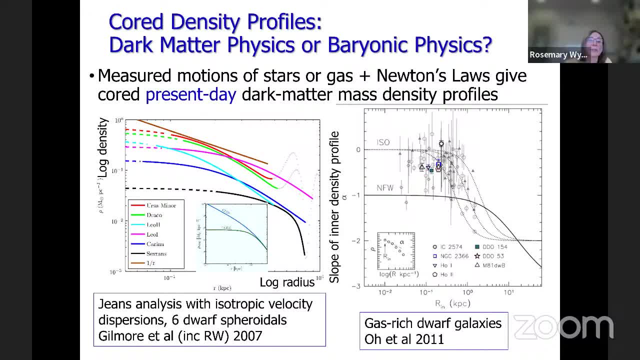 result with the assumption of isotropic velocity dispersions. so we argued that the fact that they all gave the same result suggested that that result was valid. that's the gas poor. gas rich is shown on the right hand side here. for gas rich you don't have the ammonium but you do have theист race of gas rich where it makes. 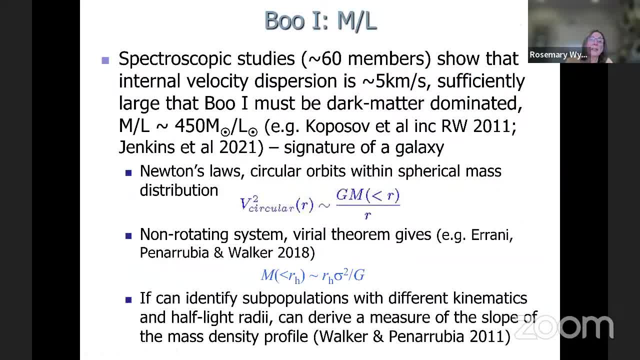 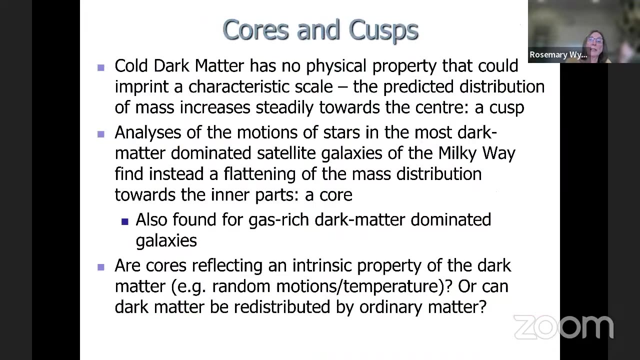 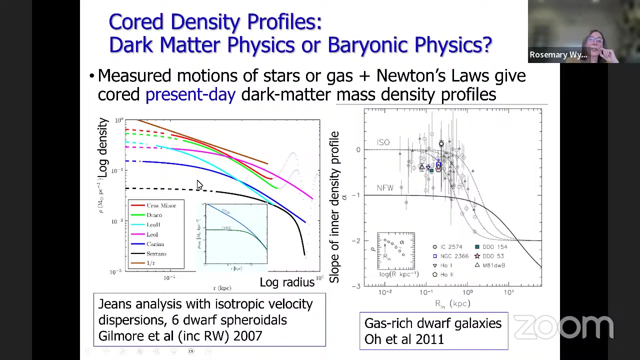 um ambiguity back here that you're just measuring one component of a velocity dispersion for gas rich. you actually use tracers that are in circular orbits or close to circular. how close they are is a source of some debate, but not very much. and here's gas rich again. this is the slope of the inner part here. 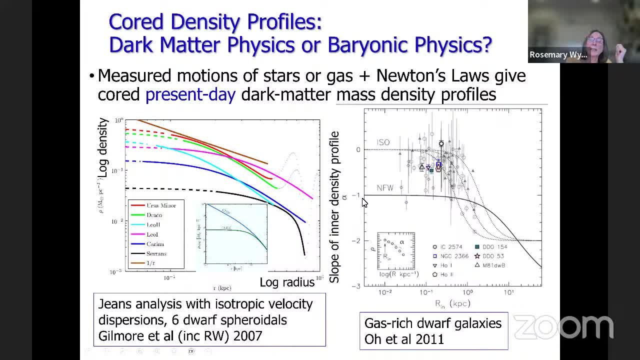 Navarro-Franken-White is down here, a core is up here and the bulk of the systems are up here, also not consistent with Navarro-Franken-White. so, assuming that this is correct, it would make sense that both gas rich and gas poor dwarfs have similar profiles. 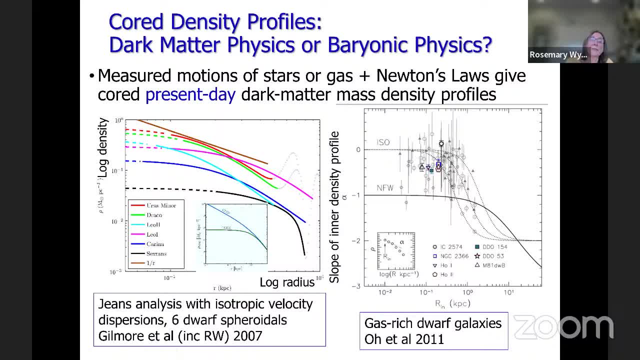 but then that leads to the fact, to the question that, okay, people said, okay, we'll accept their chord, but that's the present day dark matter distribution and maybe it's been effected by the fact that the dark matter has baryons inside, and that's what we'd like to test. we don't actually have any mass profiles for. 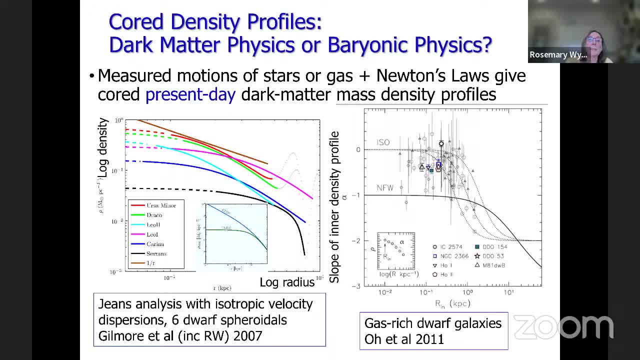 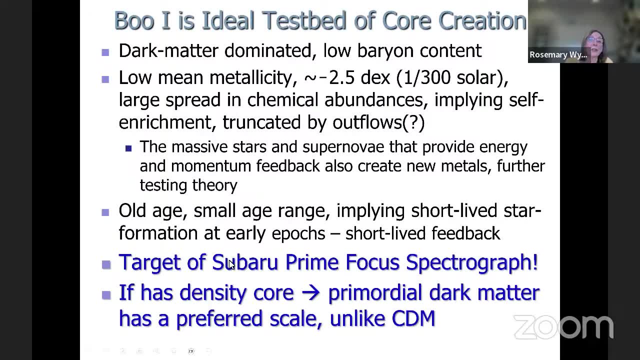 the ultra faints yet, and that's why it's really important to include an ultra faint in the sample that we're going to get with theggi nice. with the Subaru prime focus spectrograph, All we have at present for the ultra fence is 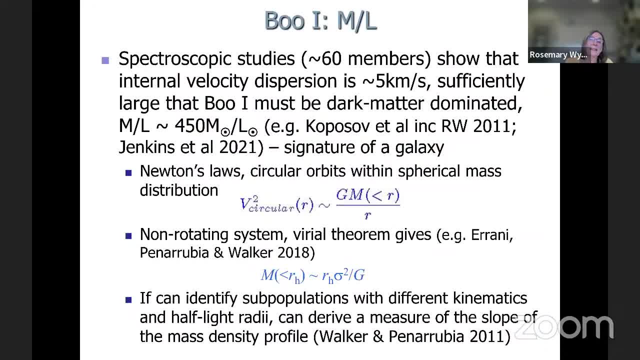 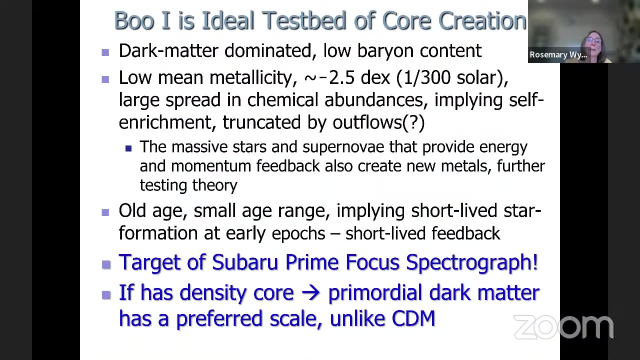 sorry, going back here, is this one estimate of the mass inside the half-light radius And that's basically the analysis here. So we don't have a detailed mass profile, but that's what we want to get And with all the data that we're going to get, 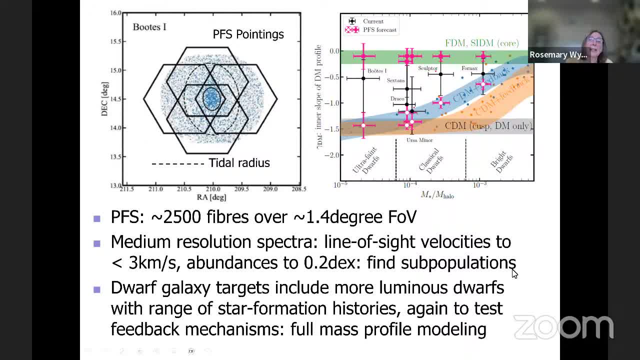 we're at least going to be able to find subpopulations in Booty's one, And we may even get enough stars, because we don't really know. I mean, I briefly went over that We know there's some stars out here. 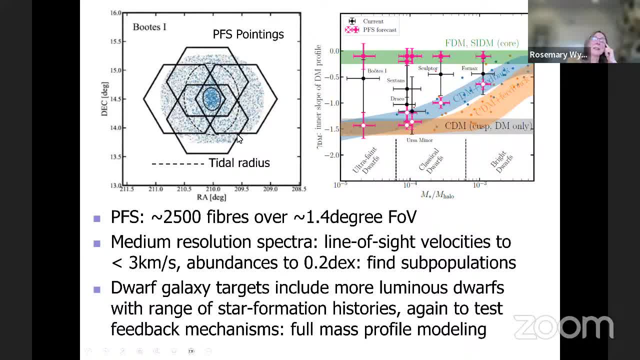 but we don't know how many member stars there are And we have enough fibers that we're just going to target everything. Okay, Thank you very much. Yeah, Thanks, Thank you. Do we have questions from the audience online? If not, 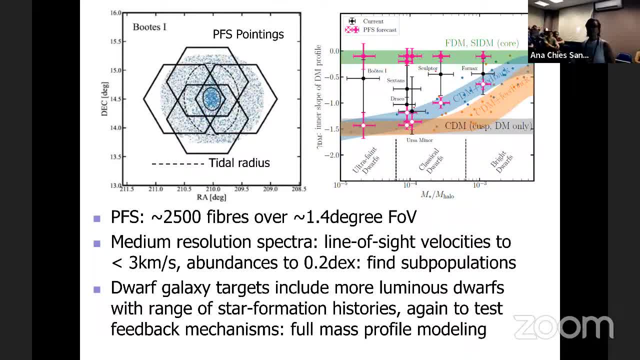 I have one question, that is, in the past years there's been lots of talk about the ultra diffused galaxies and some people say they're separate type of galaxy, but it seems they're just more of a continuum. So I'd like to hear your view on this topic. 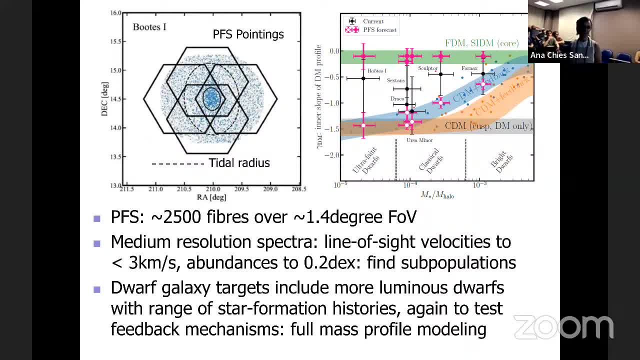 connecting to ultra faint dwarfs. How similar do you think they might be in terms of dark matter? Maybe I think that we're. we are now discovering that there's a whole low surface brightness universe that has not yet been well explored. 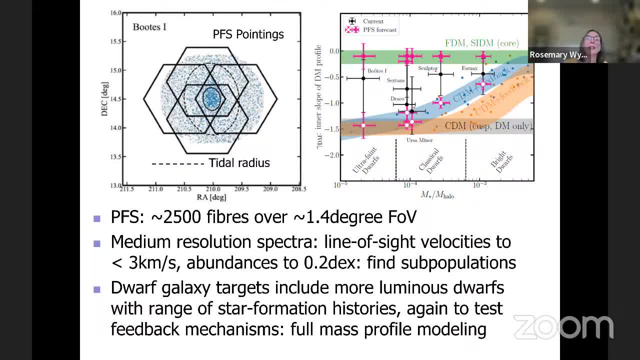 Some of the ultra diffused galaxies do seem to be in clusters and plausibly have been tidally affected by the uh, the galaxy cluster environment, And how much that has contributed to the low surface brightness is still to be determined. I think the 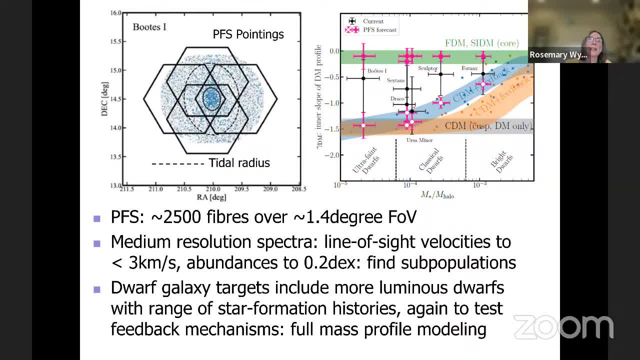 uh, whether there's a continuum in luminosity from the ultra faint dwarfs through to the ultra diffused dwarfs, I would say, remains to be seen. I think most of them that have been discovered. I think it's still true that most of them have been discovered in. 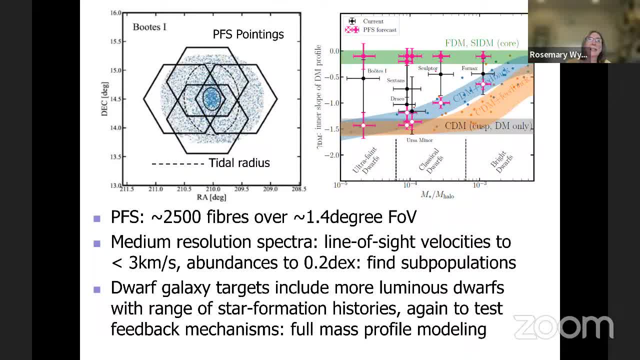 as I say, large clusters of galaxies and they do tend to be much more, much higher luminosity than these little dwarfs that we're talking about. But I think some similarities and how they formed, but they probably haven't had the same outflows that would be contributing to the low. 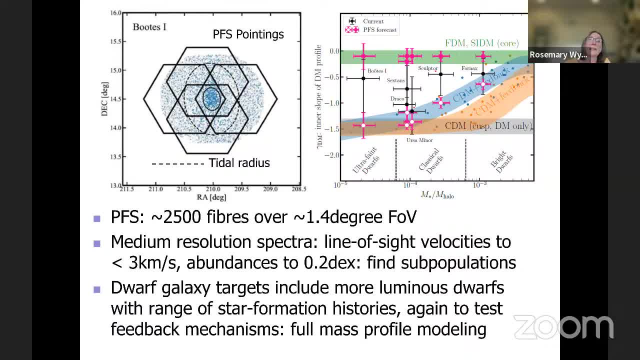 baryon content and, plausibly, the extended distribution that we saw. We see in the ultra faints. So some similarities in physical processes behind the low surface brightness, some not. I think it's a very interesting question though. Yeah, Thank you.